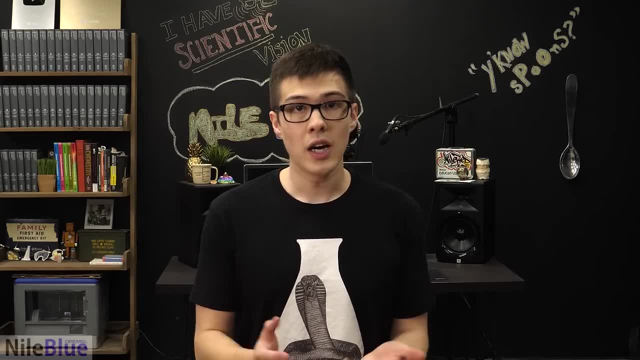 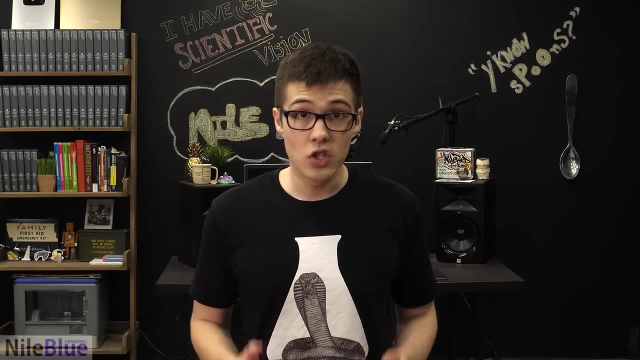 basic things like wearing goggles or a lab coat. This was kind of okay in the beginning of the channel because my audience was mostly chemists. However, the channel has grown a lot and that just isn't the case anymore, So I've decided to make a proper video dedicated. 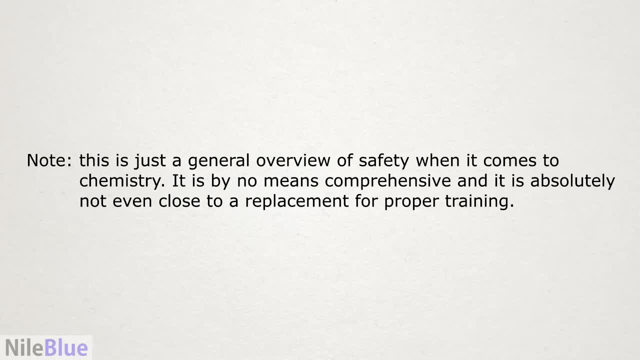 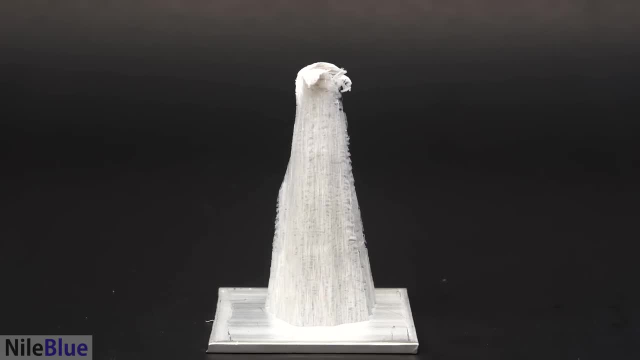 to safety when it comes to chemistry, which I think is a long time overdue. I think that chemistry is one of the most exciting branches of applied science, but in my opinion it's also one of the most dangerous. It can involve almost every hazard possible, from fire to. 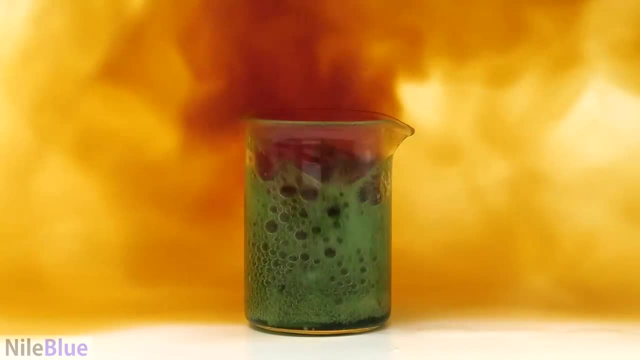 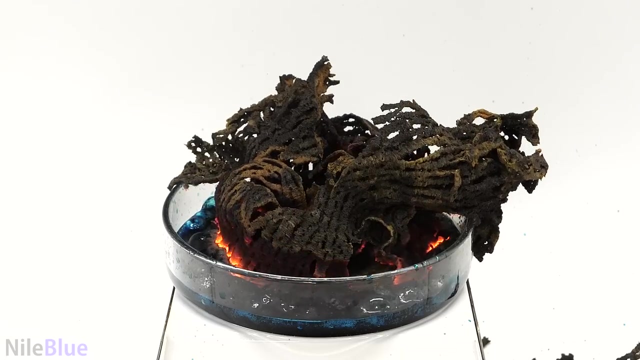 explosions, to poisons or toxic gases If you don't know what you're doing, and well, even if you do know what you're doing, accidents are going to happen. The main difference, though, is that if you're prepared, you can make them happen. 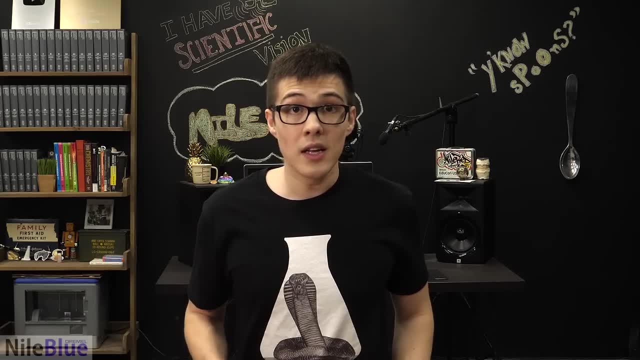 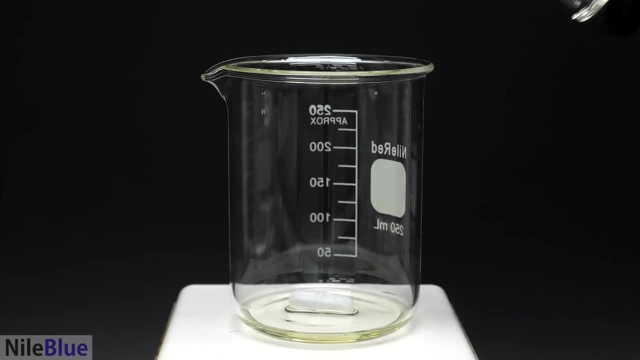 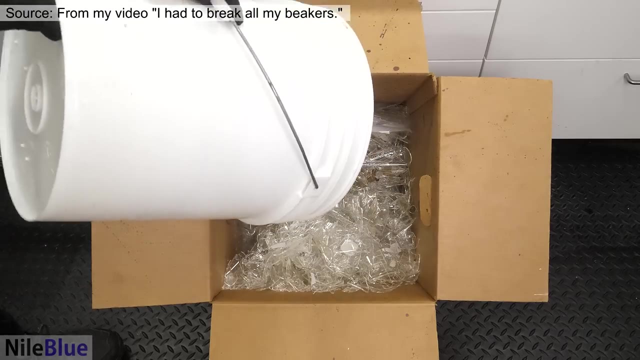 I've been doing chemistry for years and I have had many accidents, but because I took basic safety measures, none of them have been serious, Besides minor cuts from broken glass or something, I've never had a major injury and no one around me has been injured either. 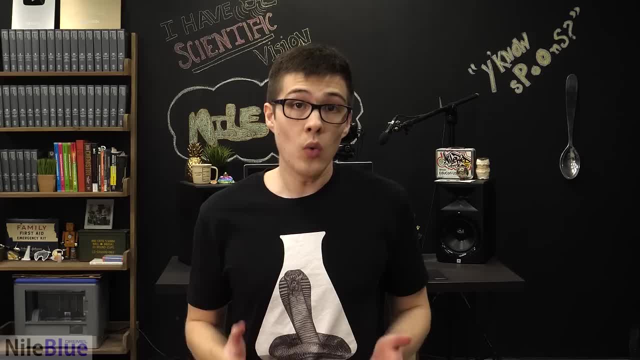 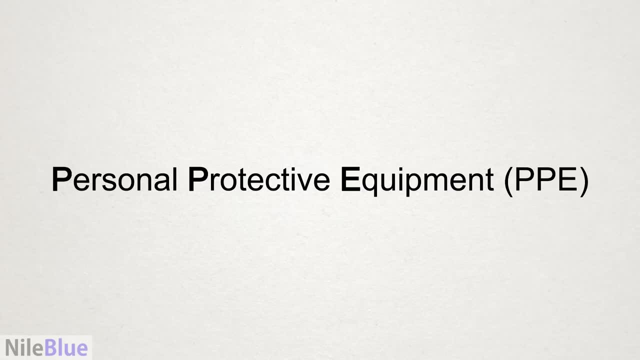 When it comes to basic safety, there are many aspects, and the lowest level of it is just what you're wearing. The proper term for this is personal protective equipment, or PPE, And the most common form of this are gloves, goggles and a lab coat. 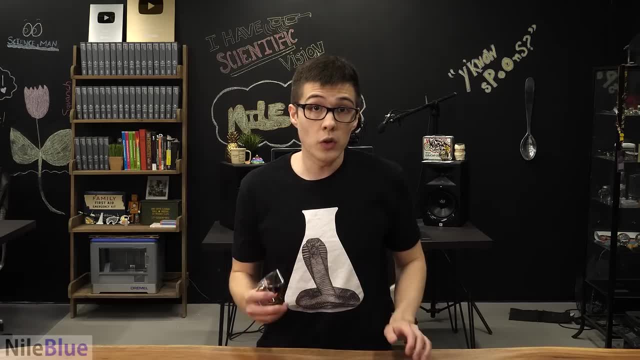 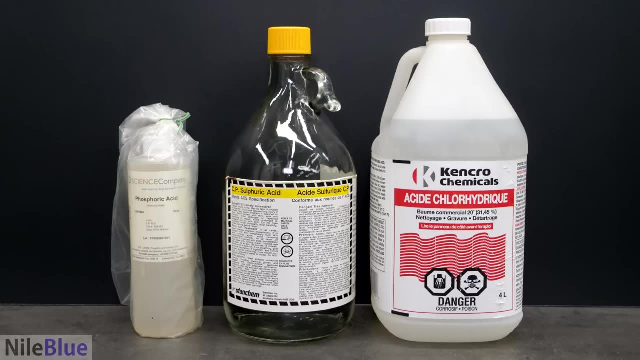 Goggles are, of course, used to protect the eyes, which are the most vulnerable part of you. There are many commonly used chemicals, like acids, that can easily and quickly blind you or at least permanently ruin your vision. Goggles are the most important barrier to this. 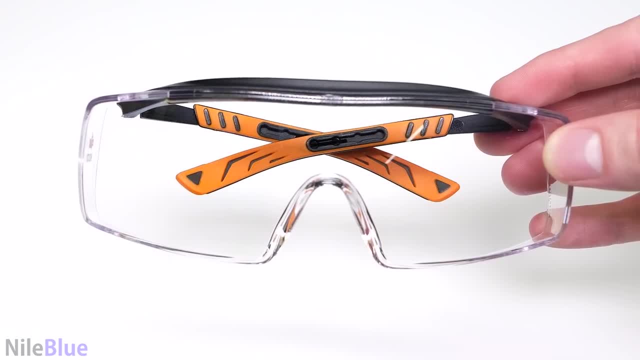 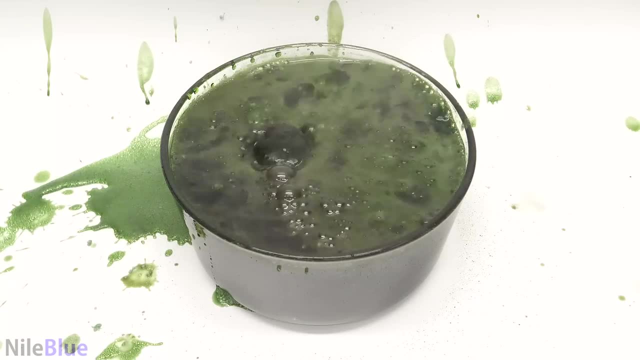 and I've personally had my eyes saved by them at least a couple times. Also, most of the time that you get something in your eye, it's because something splashed or popped and it would be completely unexpected. So for this reason, you just need to always wear goggles by default. 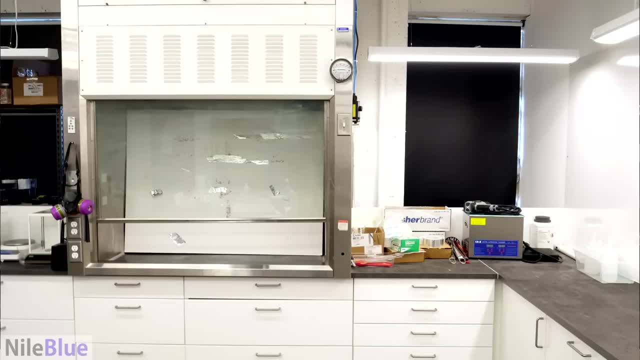 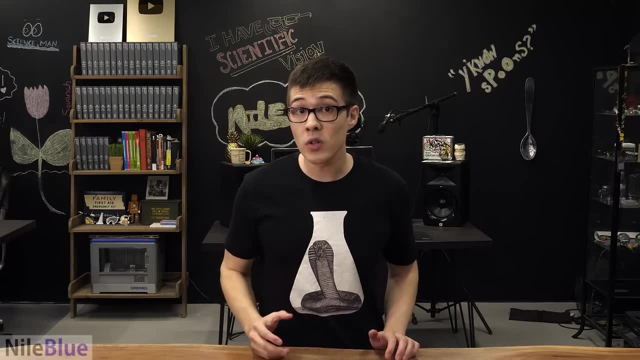 the moment that you enter the lab, even if there doesn't seem like there's anything going on. I learned this lesson when I was a lab tech about six years ago, when I was cleaning up hours after the students had left. There were just a couple things left over, and one of these things was a 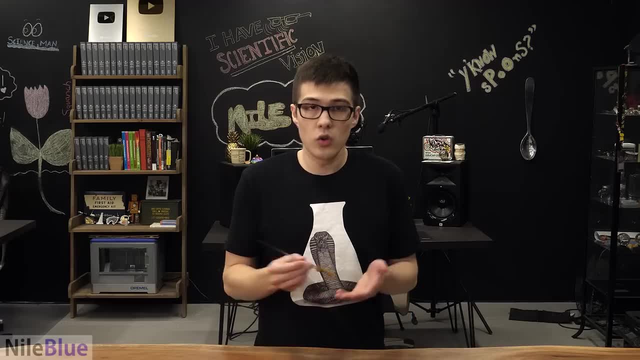 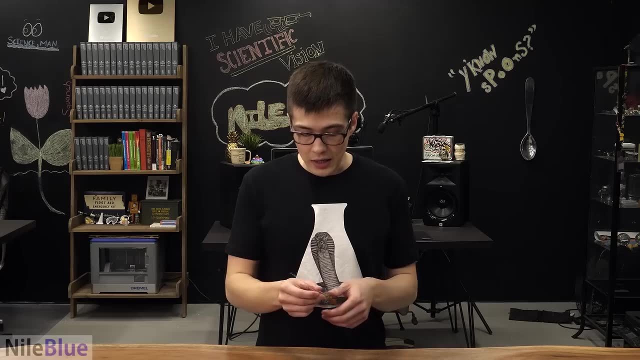 used pipette with a bulb that was still on the end. Students would always forget these, and every day I had to clean them up. For whatever reason, though, this time I tried to take off this bulb, and I don't even know how it happened, but I ended up. 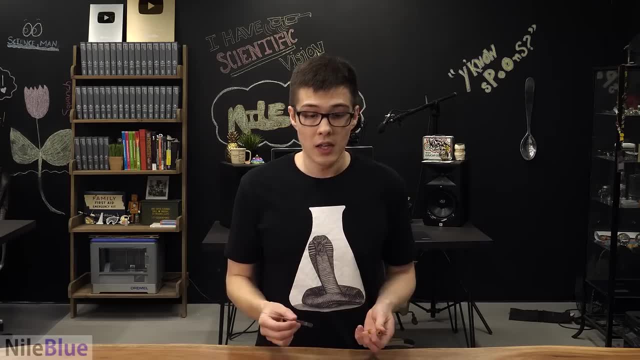 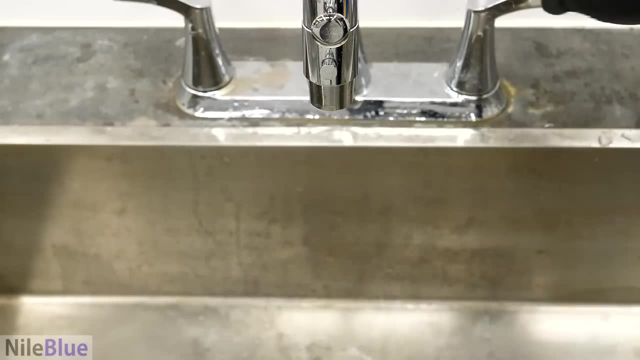 flicking the contents of the pipette all over my face. It was a mixture of strong acids and it immediately started burning everywhere except where I had my goggles. I then quickly ran over to the sink and I washed my face with a lot of water and I was fine. This all happened. 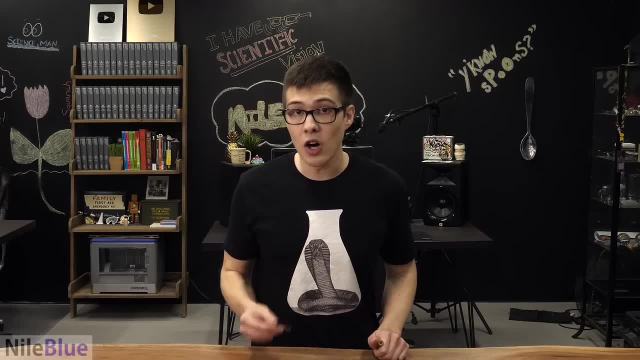 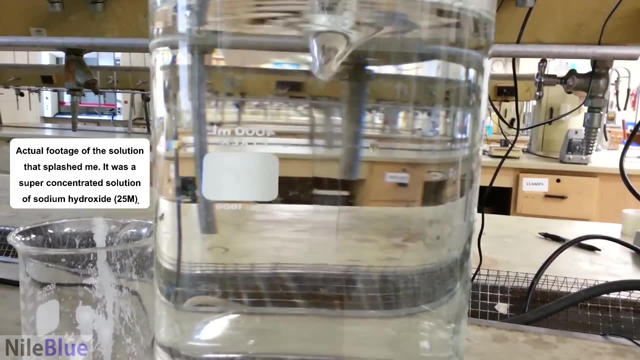 really quickly, though, and it was completely unexpected and it taught me how important goggles were. Since then, I've only splashed some of my goggles on my face, and I've only splashed something on my face. I think, once and again it was fine because I was wearing. 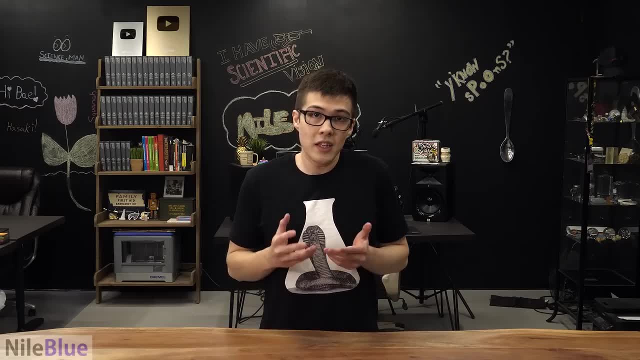 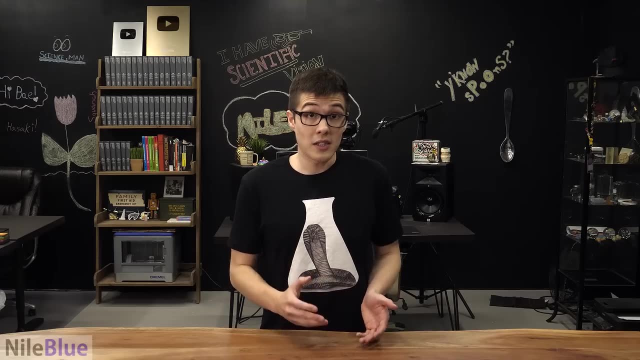 goggles. Also, your own clumsiness isn't the only thing you have to be careful of, and goggles become even more important when you're working around others. In both my accidents, no one was next to me, but if they were, it might have hit them as well, So it's important to be protected. 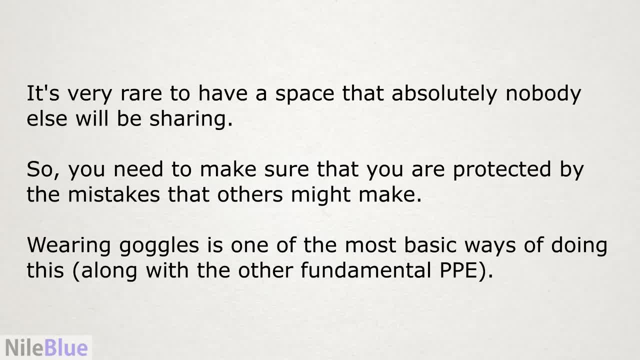 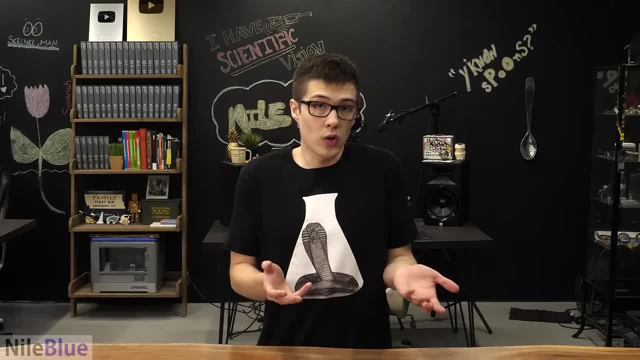 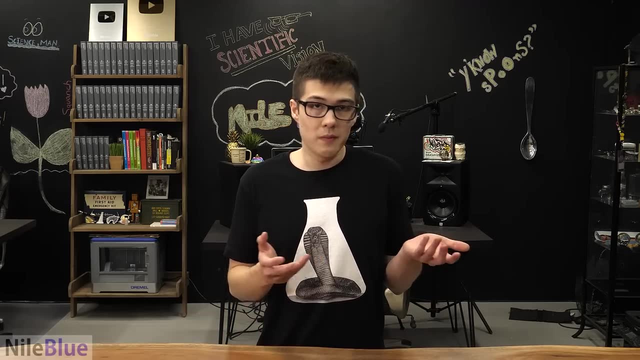 both from your own mistakes and from those made by others. Sometimes, even when you're wearing goggles, chemicals can still get around them, especially if there's a large spill, or you can also just make a mistake. For example, again as a lab tech, I once saw a student take them off just for a second or something, I think. 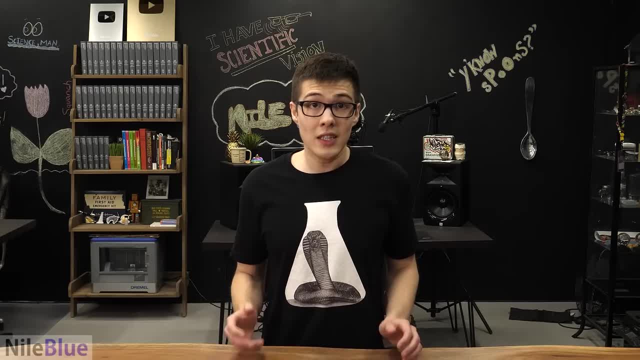 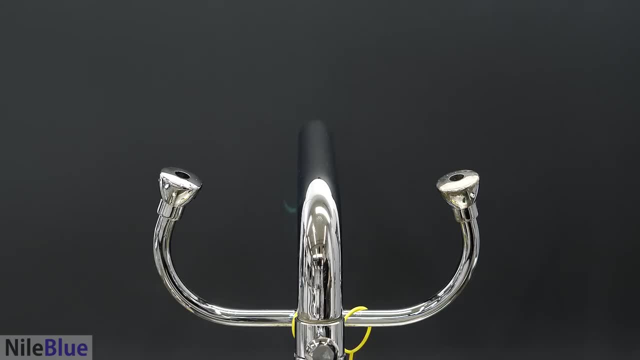 to readjust them and, coincidentally, get splashed at the exact same time Because of this, there's also another layer of safety that's really important, and this is a proper eyewash station. This makes it possible to continuously flush the eyes with water, and having one can be the 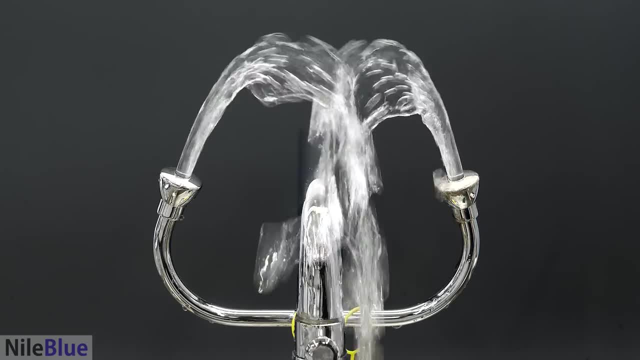 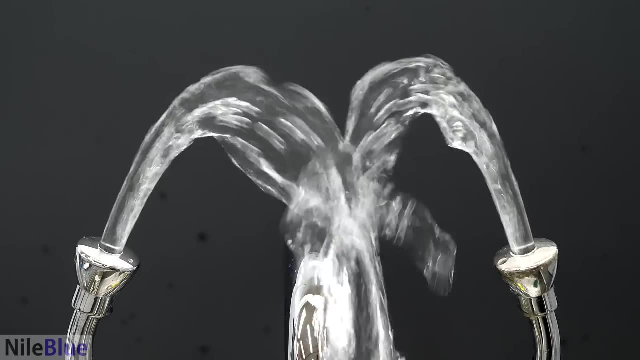 difference between permanent eye damage and being perfectly safe. So if you're wearing a perfectly fine, In most cases the damage to the eyes is directly dependent on how long it takes to wash out the chemicals. The eyewash lets you hold open both eyes and flush them continuously. 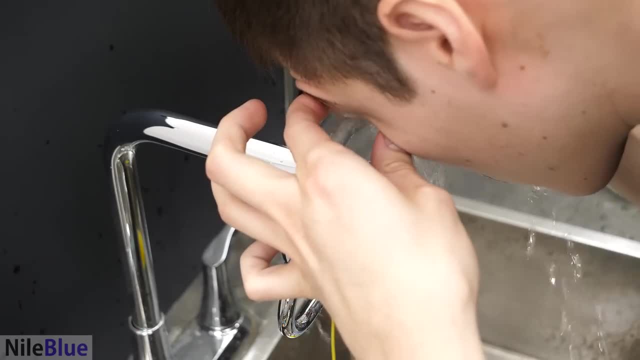 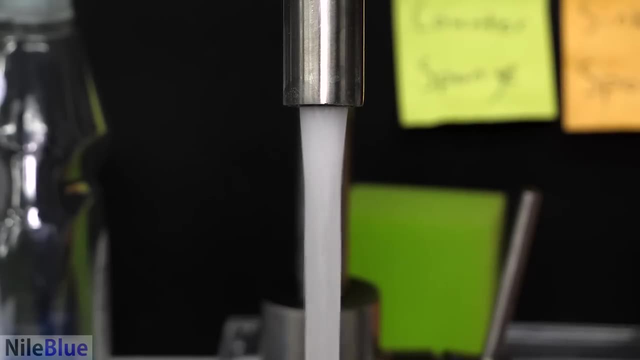 and you usually want to do this for at least something like 15 minutes. Out of curiosity, I've tried washing my eyes with a standard downward-facing tap, and it's almost useless in comparison. In an absolute emergency, maybe one of those removable taps might work for one. 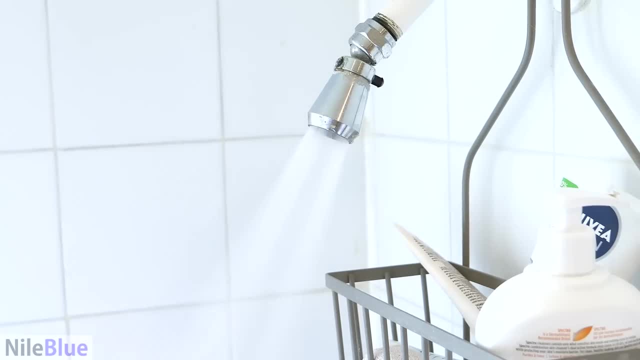 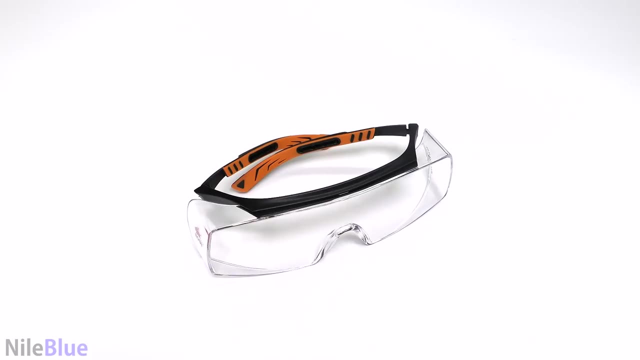 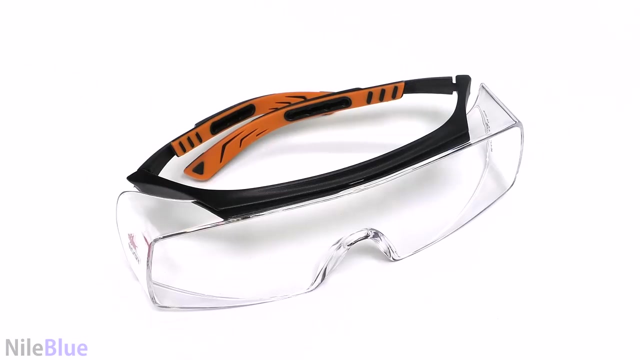 eye or a bathroom shower could work for both, but both those options are really far from ideal. With all that being said, though, the main point is that eye protection is absolutely necessary the moment you enter a lab, and there's really no exception to this. The only variable is the. 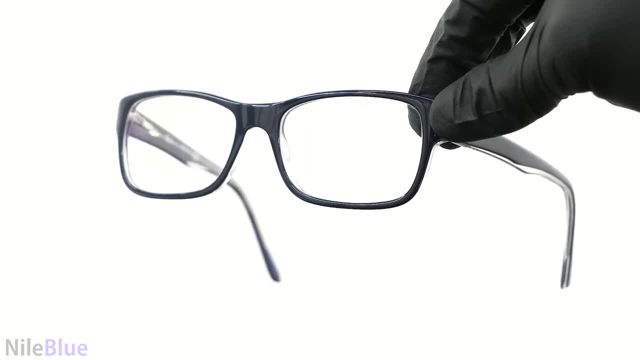 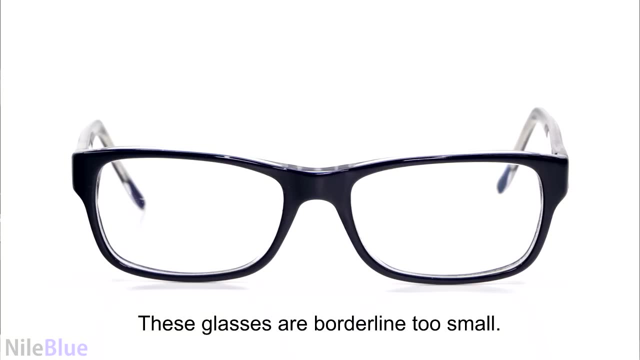 level of protection where sometimes just a pair of prescription glasses can be okay. As long as they're big enough, they generally offer enough protection from small splashes like the one I'm wearing right now. So if you're wearing a pair of prescription glasses, 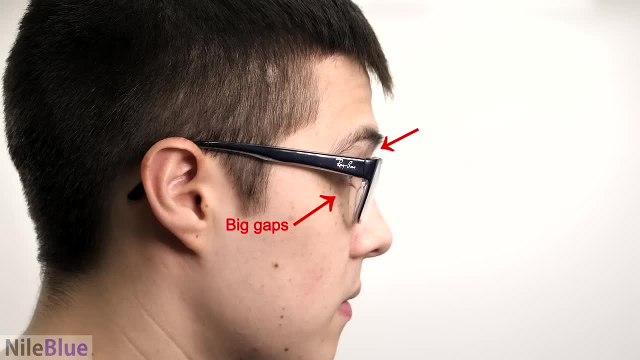 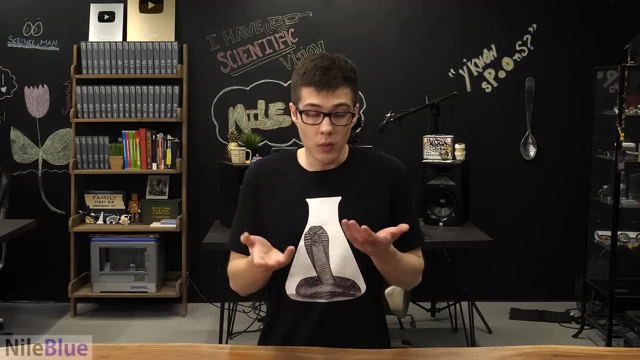 they're the one that happened to me. They don't, however, properly cover the sides and liquids can still get around them, So I only use these glasses when I'm doing something that has pretty much zero risk of splashing, For example, in a video that I posted a little. 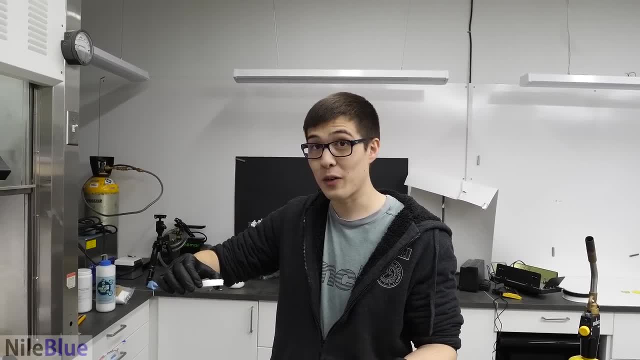 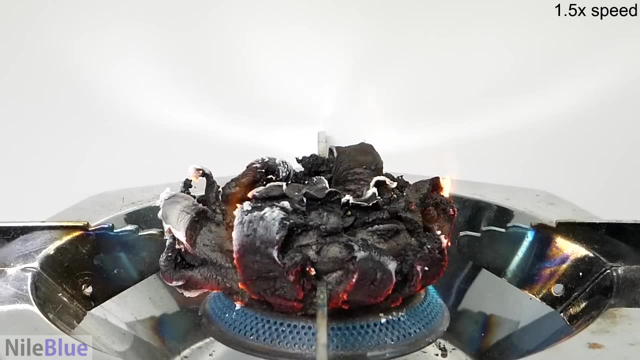 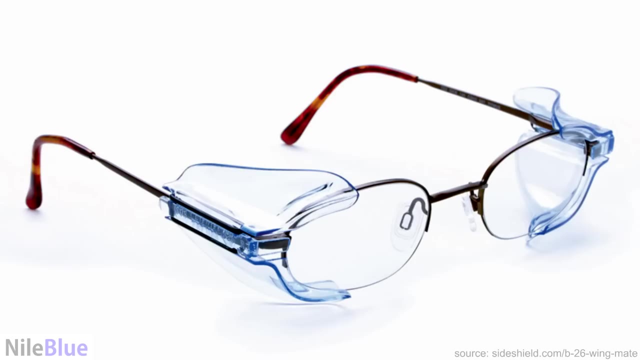 while ago on this channel, I wore my regular glasses because all I was doing was burning some tablets on a camping stove. If, however, I at any point had to use acids or even just a solvent, or if I had to touch a dirty pipette, I would have put on my proper safety goggles. In theory, 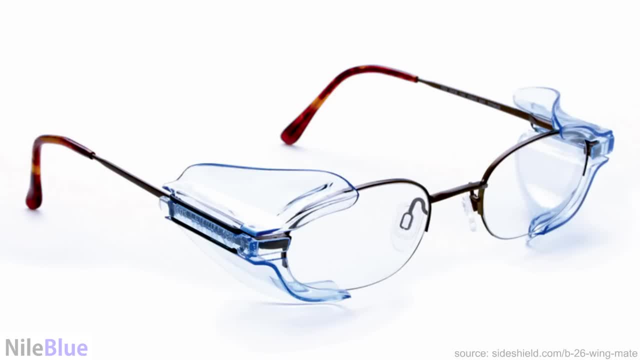 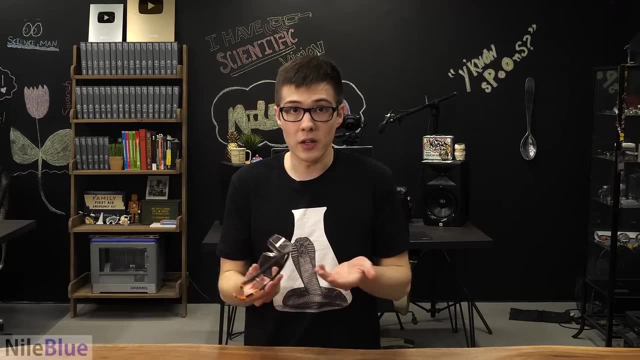 it's also possible to buy these clip-on shield things that go on the sides and below prescription glasses, but I find them kind of pointless. It's so much easier just to find a decent pair of safety goggles that are able to go over and completely cover the glasses, In my opinion. 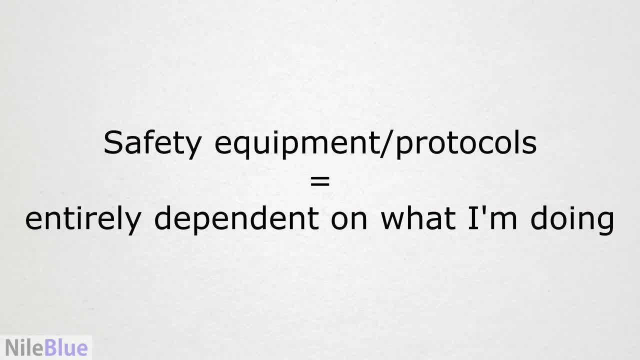 this idea of adapting the safety equipment to the particular project or environment is the best way to do things. I find it very easy to do this and I think it's a good idea to do it with a pair of safety goggles. If you're wearing a pair of safety goggles, or if you're wearing a. 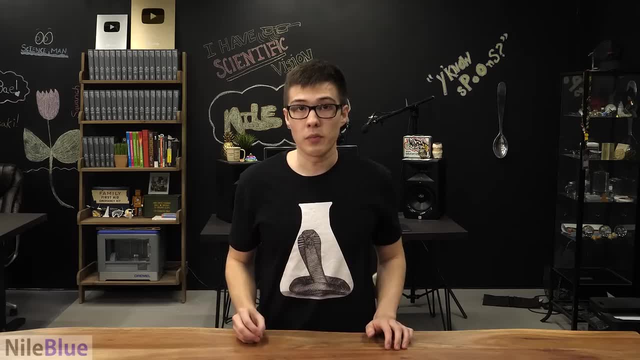 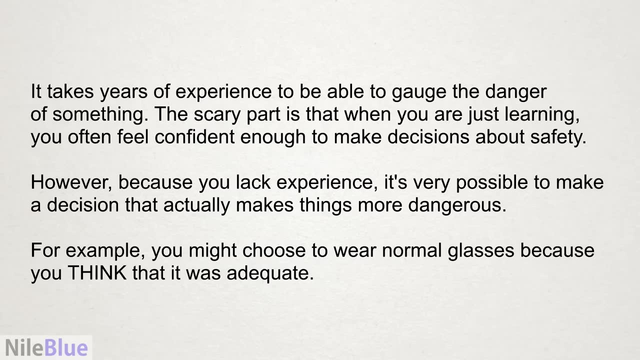 pair of gloves. I find that it's a lot safer because it means that I'm taking a much more active approach and I'm constantly evaluating the danger of what I'm doing or what I will do. However, if you try doing that without enough experience, you could be actually putting 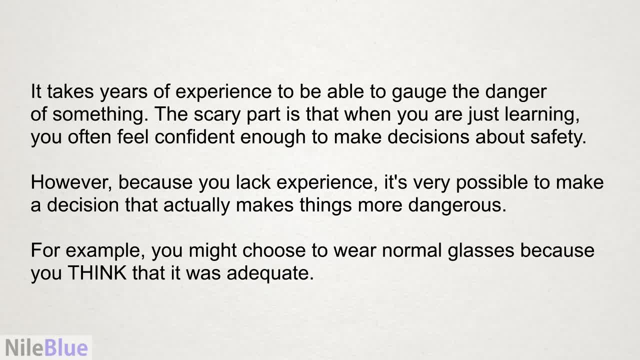 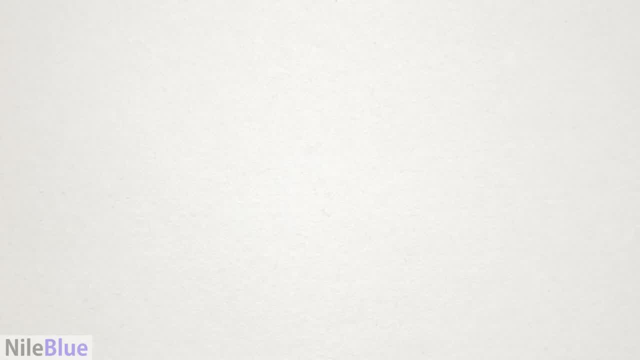 yourself in danger. So when just starting with chemistry, it's very important to do everything by the book. This means always wearing the classic PPE combo of proper goggles, gloves and a lab coat. For gloves, the most common ones are: 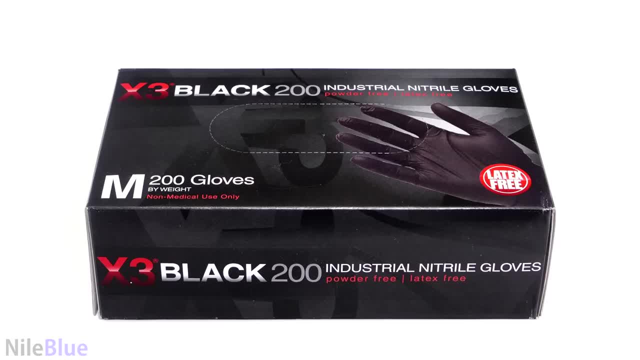 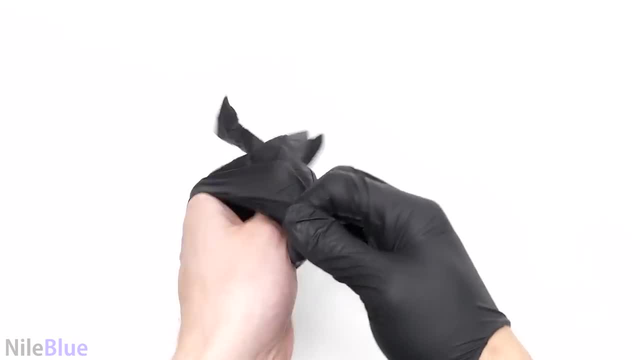 either nitrile or latex, but nitrile is usually better, because a lot of people have allergies to latex. When using gloves, though, they don't just magically make everything safer and there are still a bunch of safety precautions that need to be taken. For example, they protect your hands. 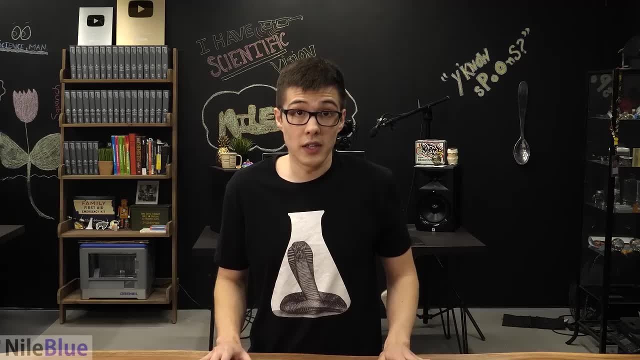 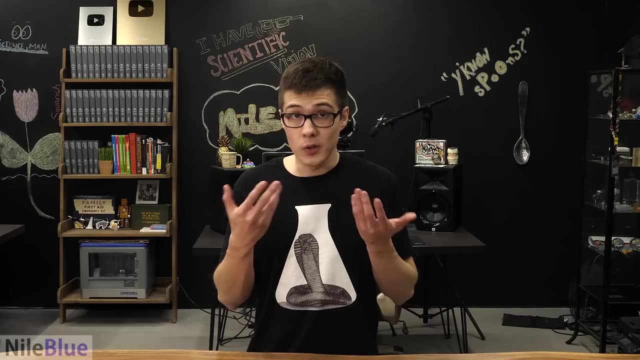 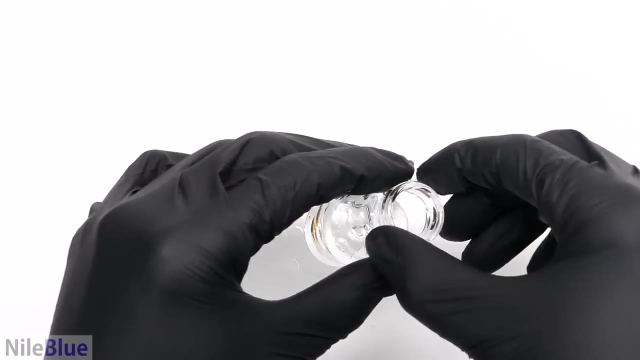 but they're also a very easy way to contaminate other things, So it's important to never leave a lab if you're still wearing gloves or to touch things like a phone, your face or clothing. It's also important to take the gloves off after they've been contaminated, because they don't 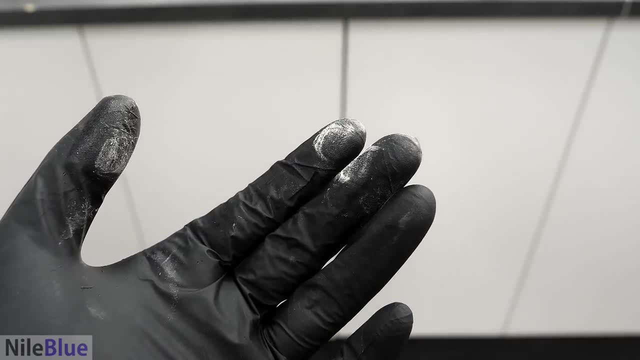 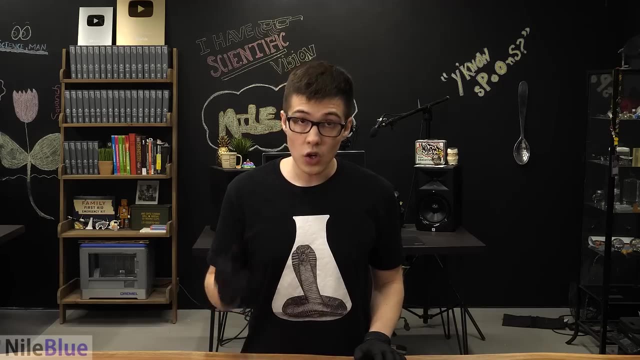 offer unlimited protection. A lot of chemicals are able to soak through them, and just leaving them on would make wearing them kind of useless. Taking the gloves off is also something to pay attention to, because if it's not done properly, it's pretty easy to accidentally touch your skin. 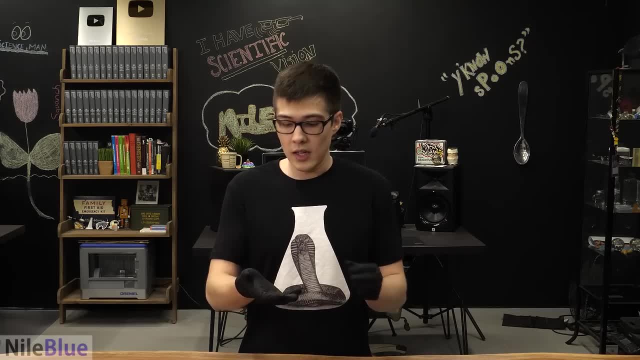 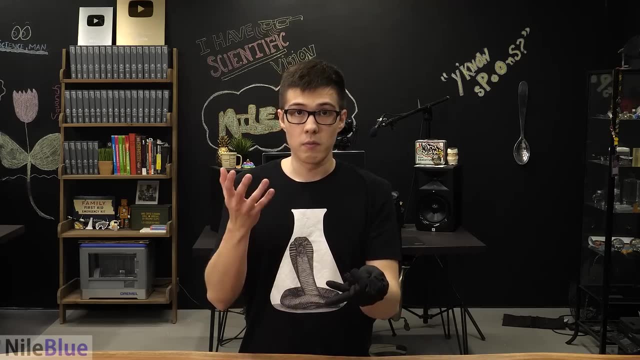 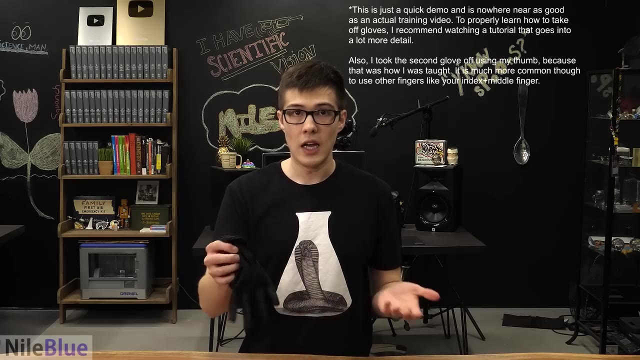 and to get chemicals on it. So the proper way is to first pinch the glove like this and to pull it off, and then, with your clean hand, you can now put it under the glove and pull that one off, and that's it. For most basic work, I just use these nitrile gloves. 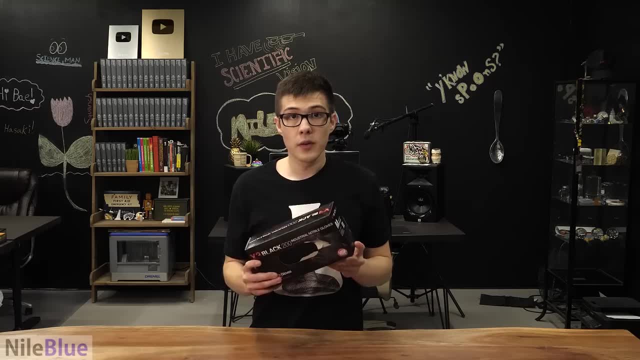 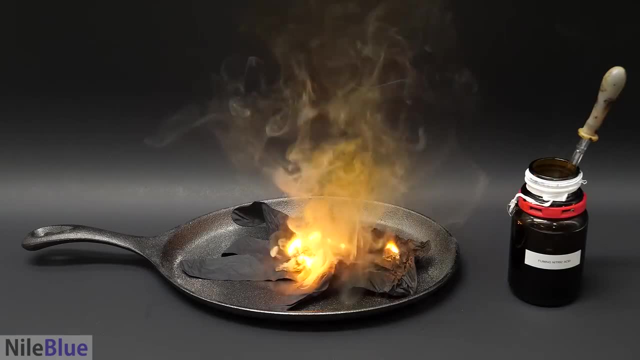 but it's always important to be aware of what the glove material is compatible with. For example, in a video that I made a while ago about nitric acid, I showed that when it's pure, it can light nitrile on fire. 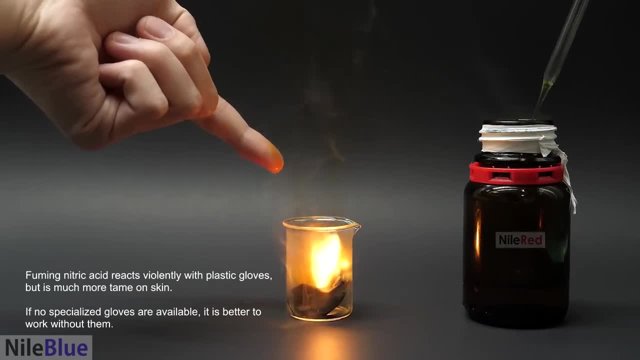 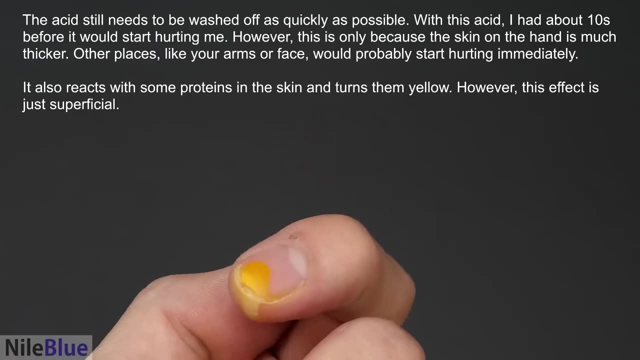 I also showed that it didn't react or do much to skin, so in this case it was safer to not use any gloves at all. However, there are other materials, like some vinyl gloves, that I could have safely worn. With enough time, most chemicals and solvents will eventually make it through a 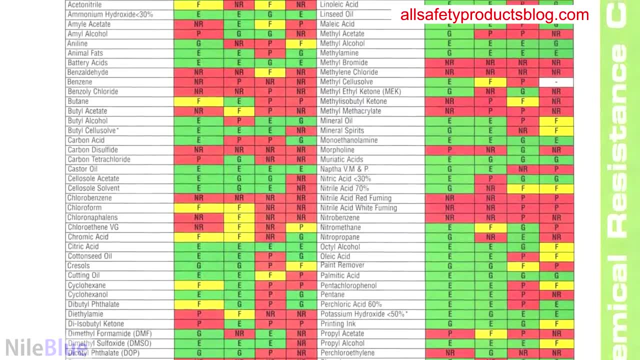 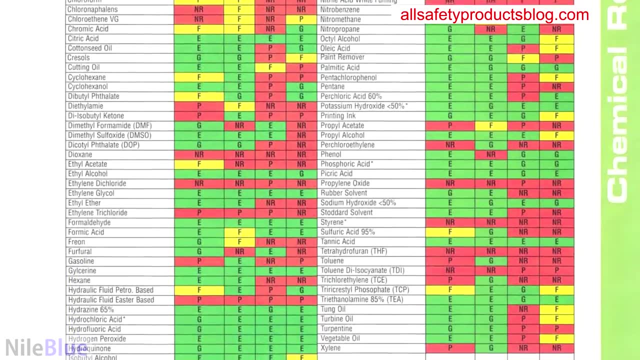 glove, but some of them can easily penetrate certain glove materials and it means that, depending on what you're using, it might not actually be doing very much. So, again, it's important to make sure that the glove that's being used is safe and that it's not going to. 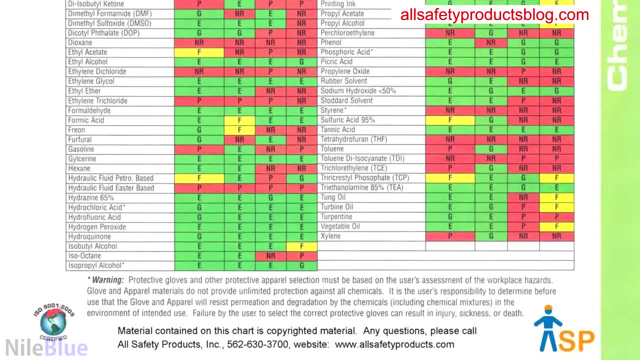 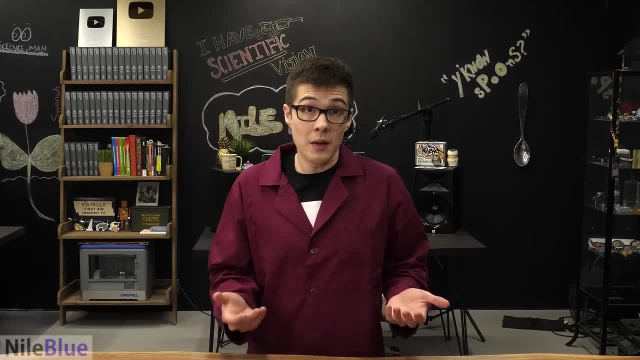 be used is appropriate for the work that's being done. Now. the last thing in the classic PPE combo is the lab coat and clothing in general. The lab coat is a good way to protect the arms and it also just stops chemicals from getting on clothing and then you leaving the lab with. 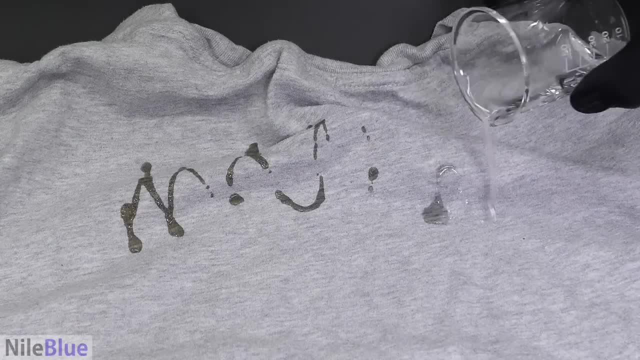 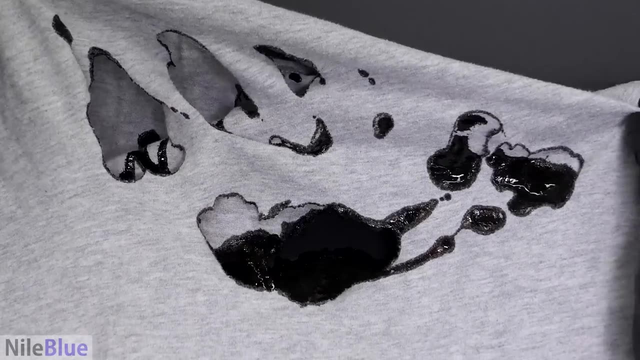 them on you. It also just protects clothing in general, because a lot of chemicals, especially acids and bases, tend to make holes and can destroy whatever you're wearing. Lab coats are also usually more resistant to the sun, so it's important to make sure that you're wearing a. 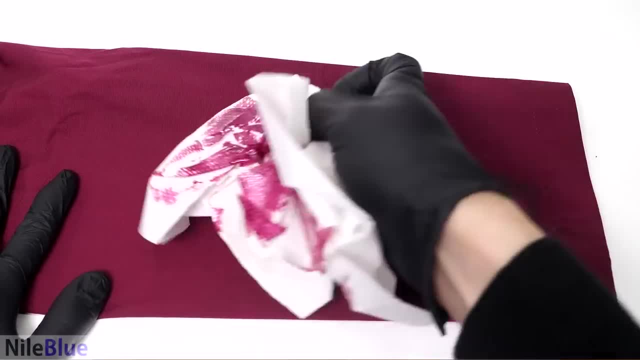 T-shirt. If you're wearing a T-shirt and you're wearing a T-shirt and you're wearing a T-shirt, you're resistant to fire and chemicals and if there's an emergency they can be taken off much quicker. This is important because if, for example, you were wearing a T-shirt and then 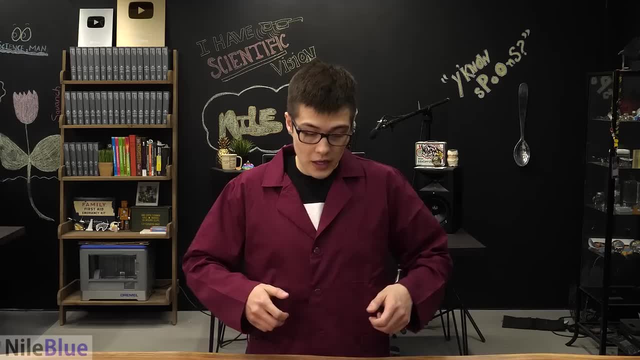 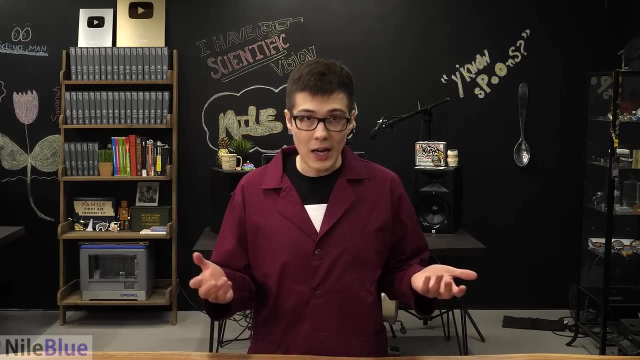 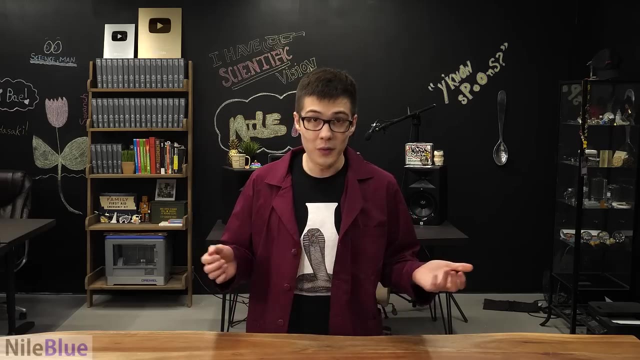 you spilled acid all over yourself. to take the shirt off, you'd have to pull it up over your face, which isn't ideal, Or if you were on fire, I would just say: good luck, even getting the T-shirt off. A lab coat, however, can just be taken off in seconds and you don't have to wipe it over. 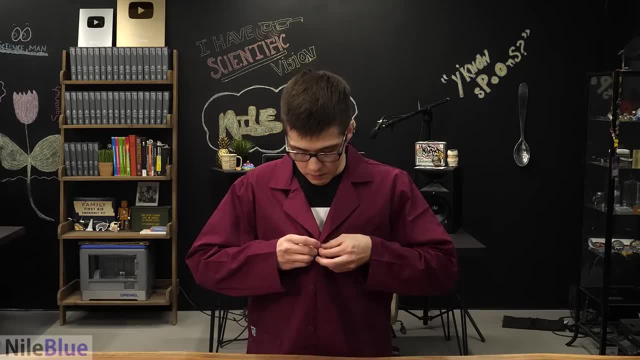 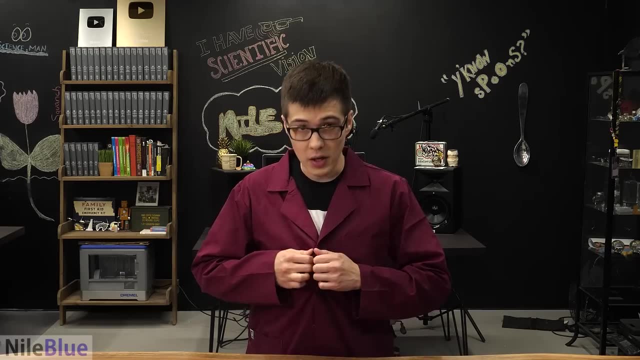 your face to do it. The one that I'm using in general is a T-shirt, and it's a T-shirt and, in particular, has these buttons, but I'm not the biggest fan of this and I much prefer those, the variety that use those snap-on things that you can just pull and instantly take them all off. 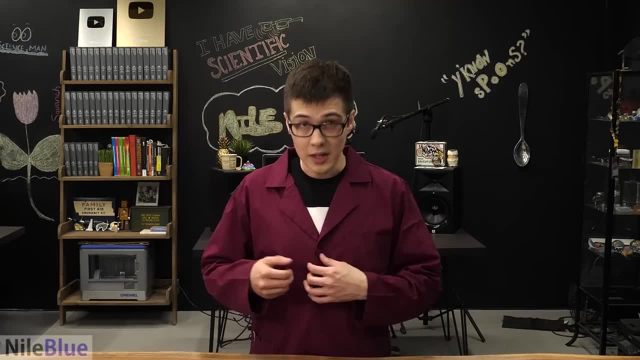 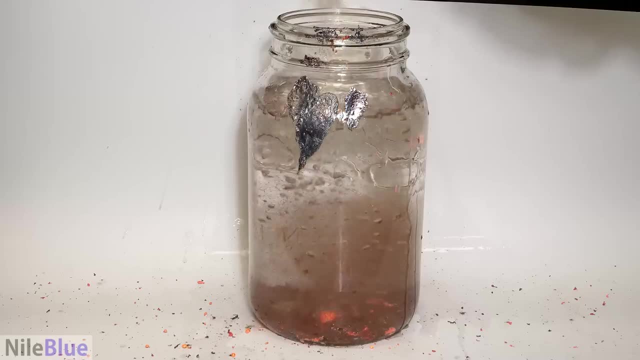 For most cases, the buttons are fine, but in an emergency, especially if you're panicking, you might fumble with the buttons and it could be a problem. In the case of an absolutely massive spill, the lab coat probably won't be able to stop everything. This is why, like with 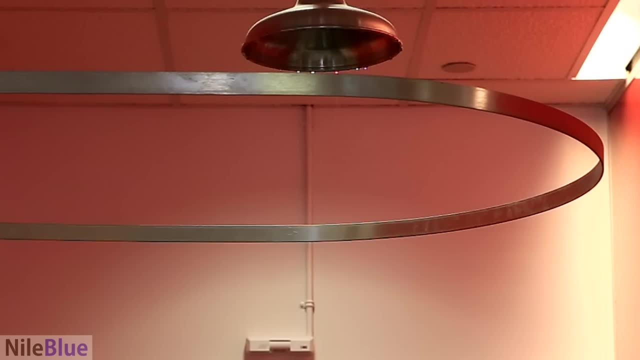 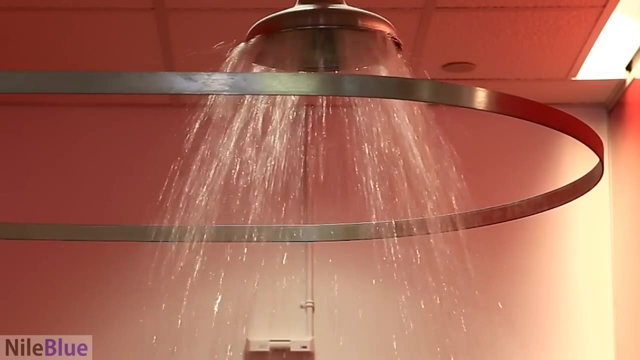 the goggles, there's usually a second measure in place, and this is an emergency shower. When the handle is pulled, it dumps a lot of water and you can wash your entire body and strip off all the contaminated clothing at the same time. Most lab coats are made of a mixture. 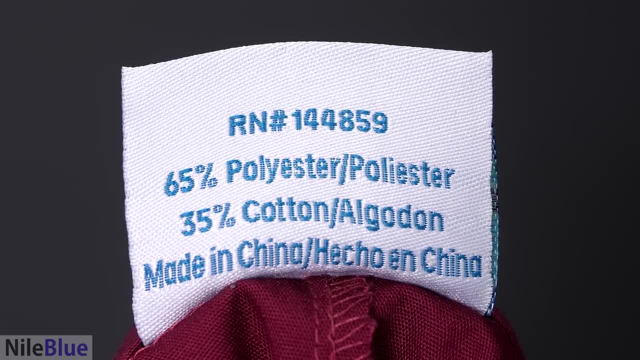 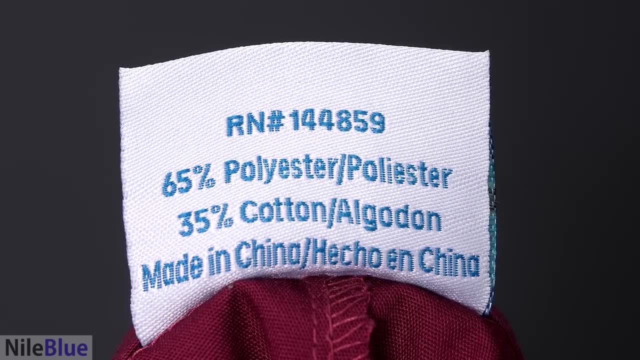 of polyester and cotton, which offer good protection for most general lab work. However, they aren't great when working with a lot of fire, because polyester and cotton are themselves flammable. Several years ago, though, some combination of polyester and cotton were used to 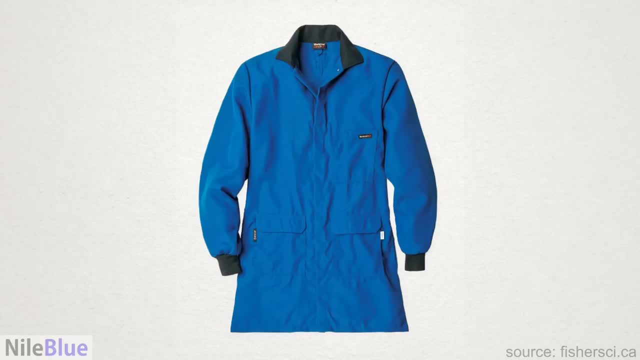 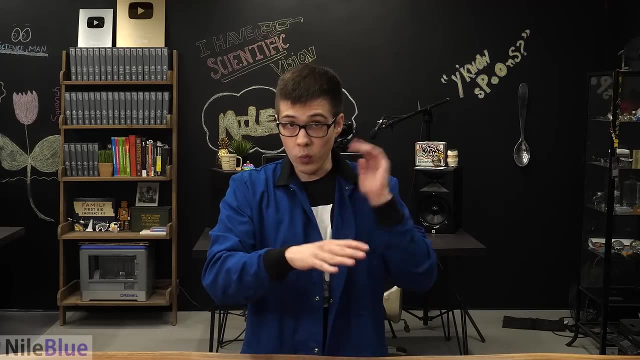 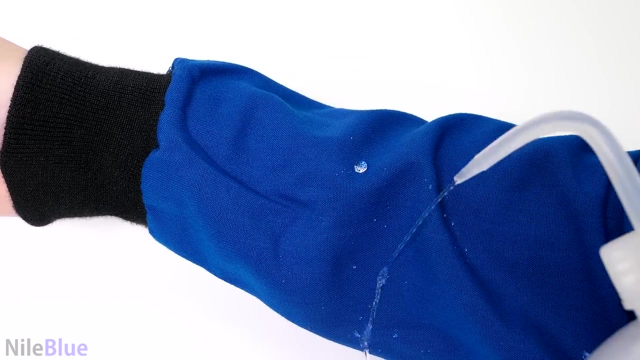 become available and I decided to buy some to replace my old, crappy ones like this one here, which I really hate. These new ones are way fancier and they even offer liquid resistance, so when things hit it, it just beads up and rolls right off of it, In my opinion. 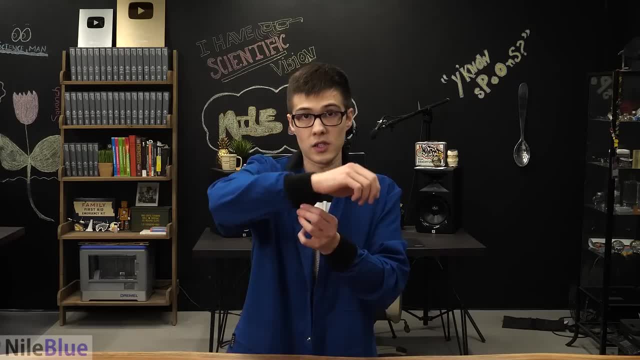 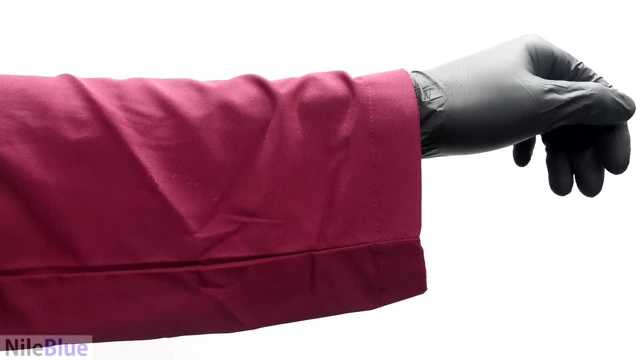 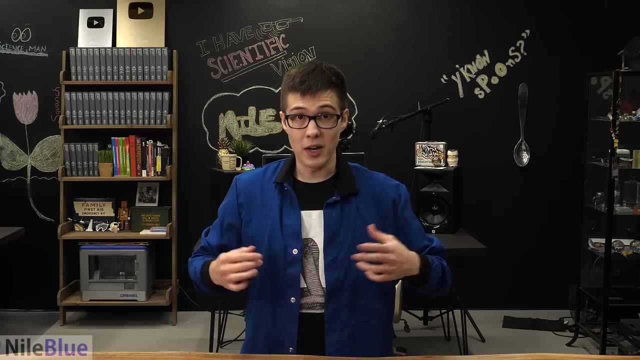 they also just look way better. and they also have these wristbands so that you don't just have a dangling sleeve that will collect and soak up chemicals off the table. And they have these snap-on buttons that I was talking about, so they're way easier to pop off. 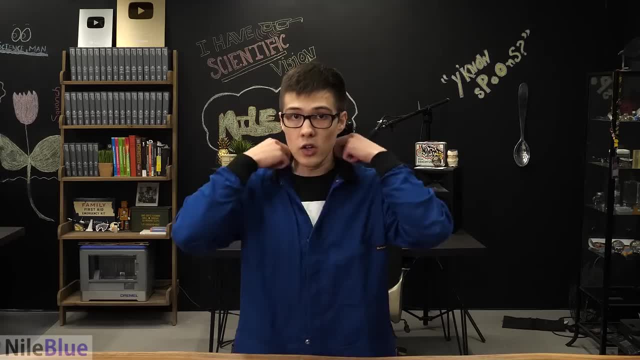 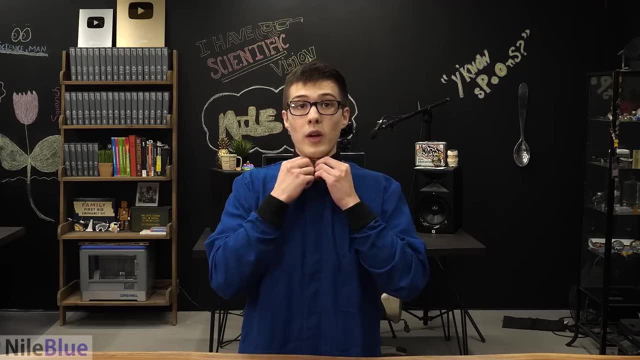 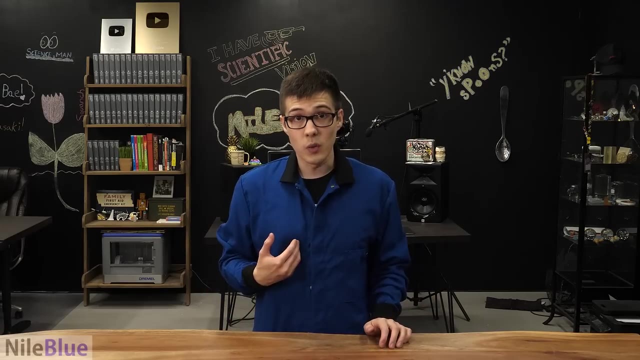 and you- yeah, you don't get stuck with all those buttons. It also goes much higher than a lot of typical lab coats, meaning that you get protection, obviously all the way up to your neck, but that really depends on what you're doing. The only issue with them is well, cost, and this one. 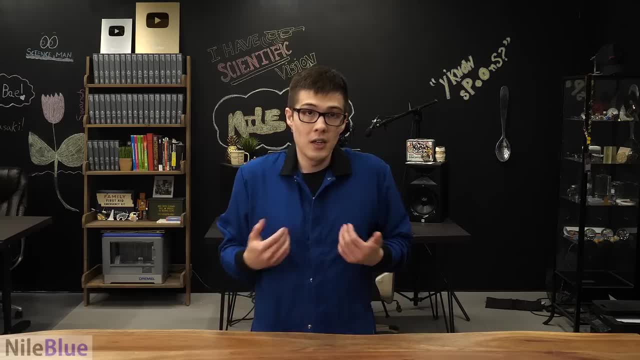 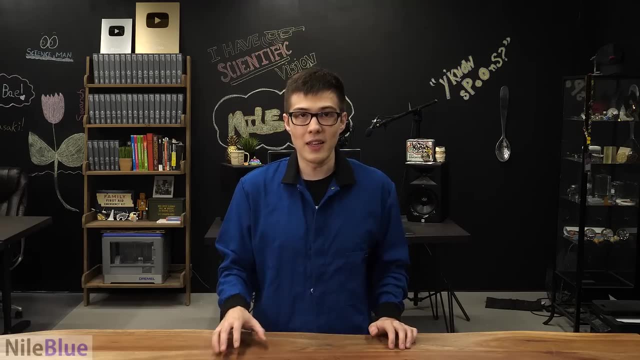 was almost 10 times more expensive than the regular one. In my opinion, it was worth it, but it's pretty hard, and it's also pretty hard to justify paying that much Again, though, with all that being said, the main point is that, like goggles and gloves, 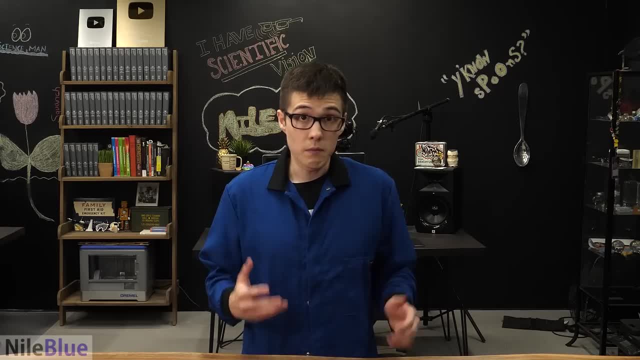 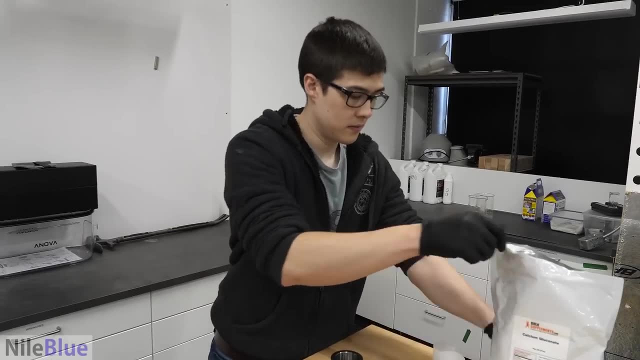 lab coats are also an active measure. So before and during each project, I'm always thinking about what is appropriate to be wearing. For example, again in that video that I mentioned earlier, I wasn't wearing a lab coat. However, this wasn't just negligence or something. 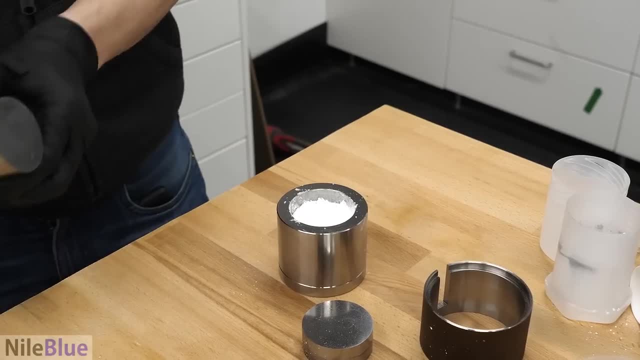 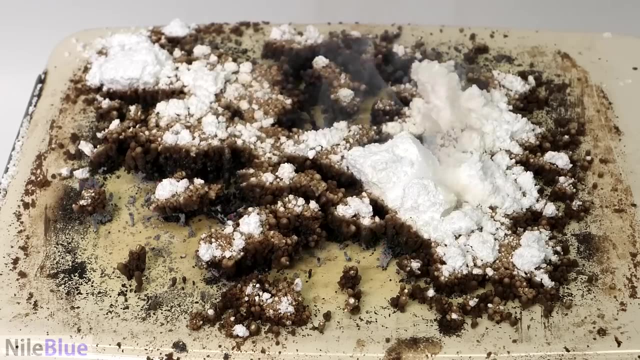 and it was because I just didn't need one for what I was doing. There was zero risk of splashing, and what I was making was almost the same as wood ash, and it was completely non-toxic. One thing to keep in mind, though, is that the ability to go completely without a coat 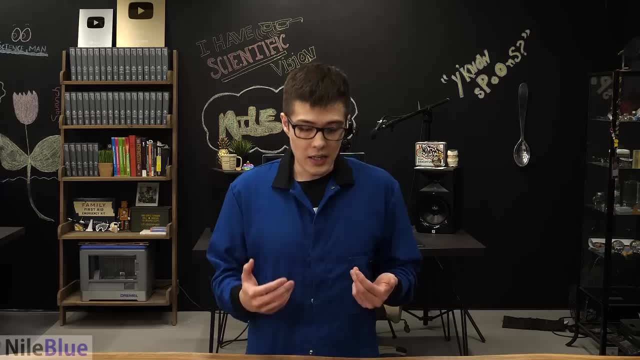 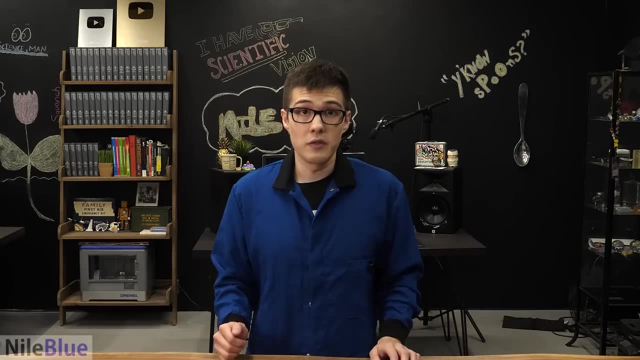 is a bit unique to my situation. This is because I'm the only person that works in this area. If it were a shared space with other people, that was not something that I could have done. Also, it was one of the few projects that I've ever done. 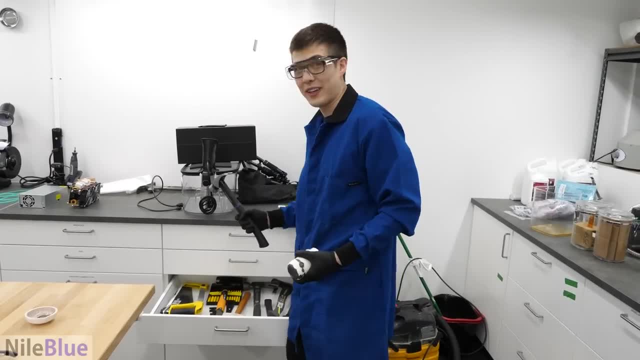 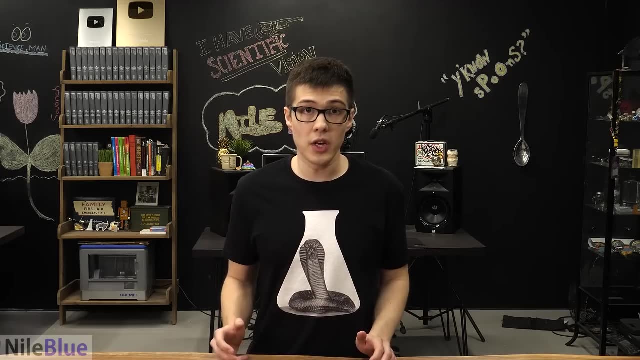 that a lab coat just wasn't needed for and in other projects you are almost definitely going to see me with one. Now, besides a lab coat, and in terms of clothing and attire in general, there are a few fundamental rules, Just like any industrial workplace. you can't just wear. 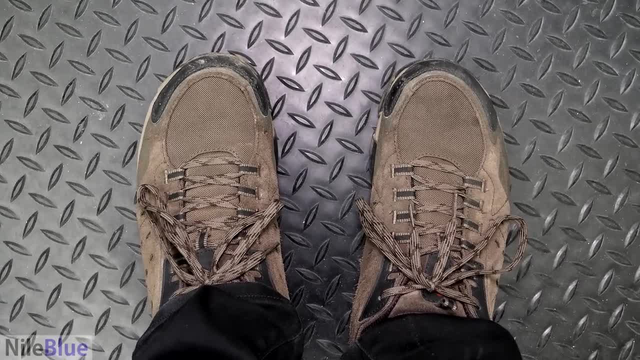 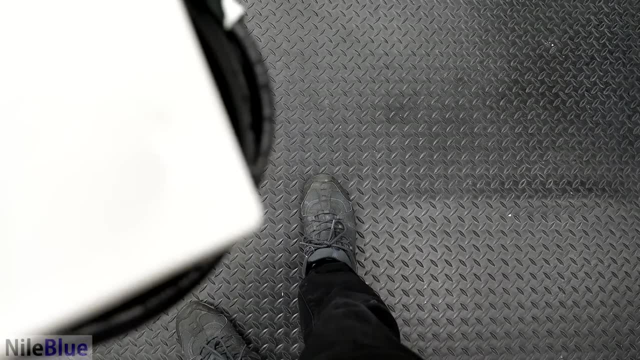 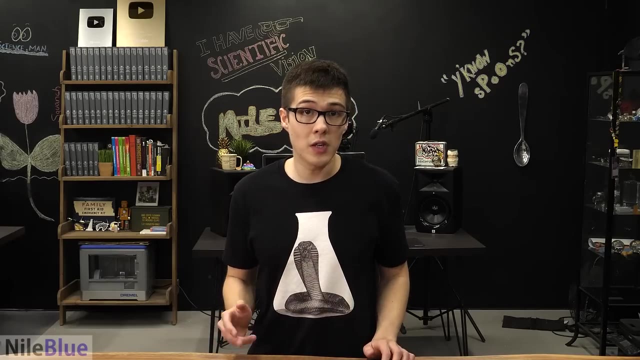 something like sandals, and the feet have to be fully covered. This is mostly to protect them from chemical spills or splashes, but it also protects them a bit if you were to accidentally drop something like a hot plate. It's also important to completely cover the legs and to never wear something like shorts. 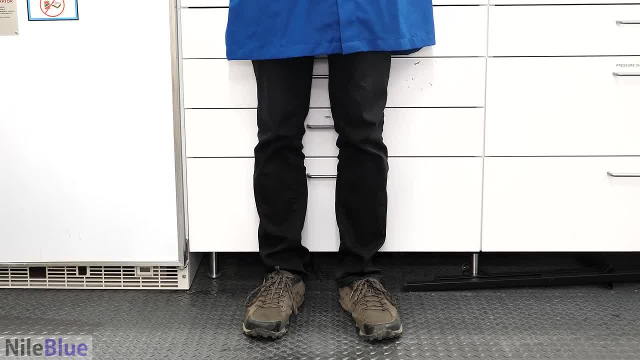 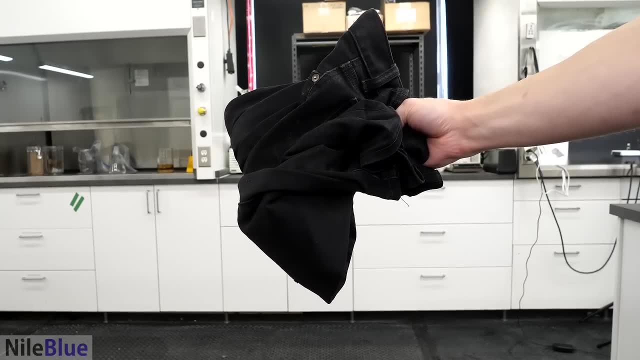 This is because the lab coat doesn't go all the way to the ground and you need to protect your legs from spills and splashes. For this reason, I actually have a pair of work pants that I keep in the lab, just like the lab coat. Both these pants and the lab coat also get washed often. 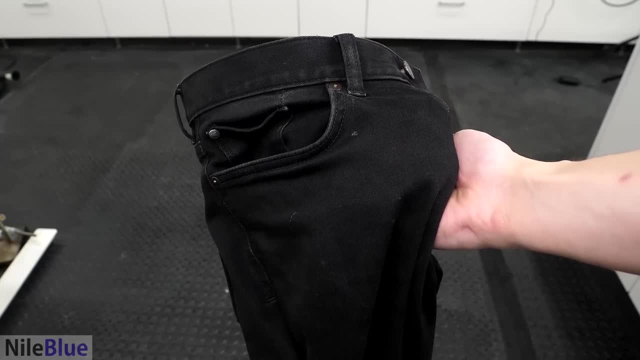 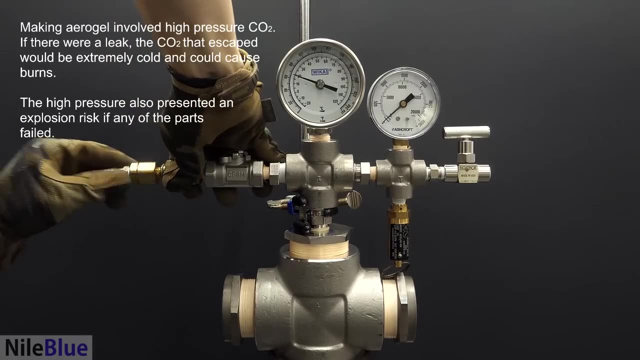 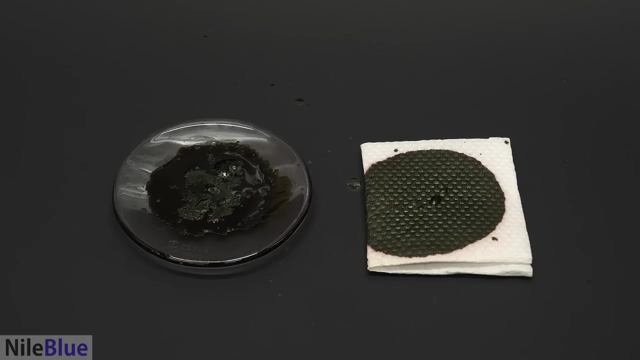 to make sure that they don't just become full of chemicals. But anyway, with all that being said, these are just some of the basic guidelines to follow. With more experience, projects tend to get more complicated and dangerous, and different PPE and protocols are usually required, For example, for some things. 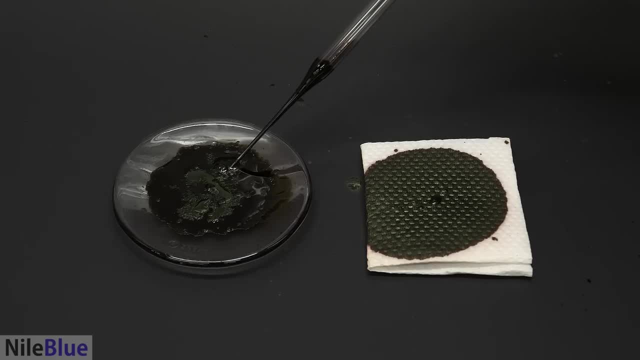 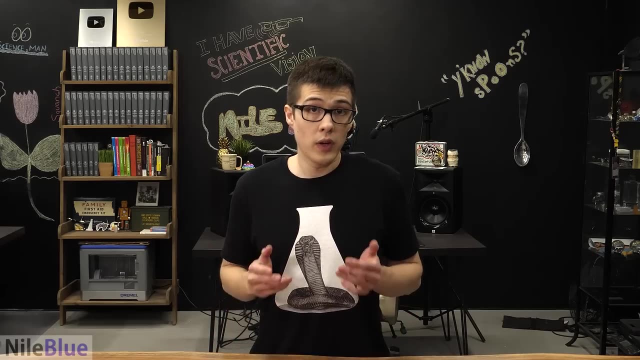 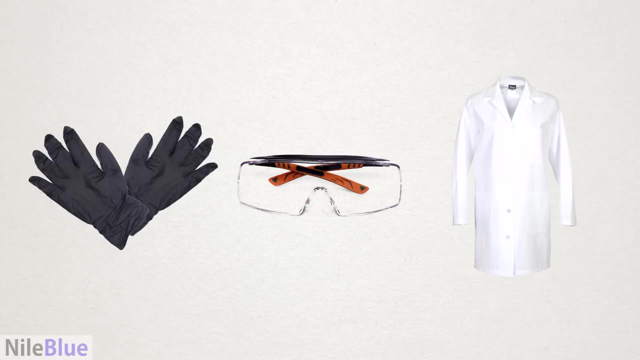 it might be necessary to wear a full face shield, specific gloves or specialized goggles. So, again, an active approach must be taken for each new project or task. Now, as I mentioned earlier, PPE is just the base layer and it offers a foundation of safety, Arguably the most important. 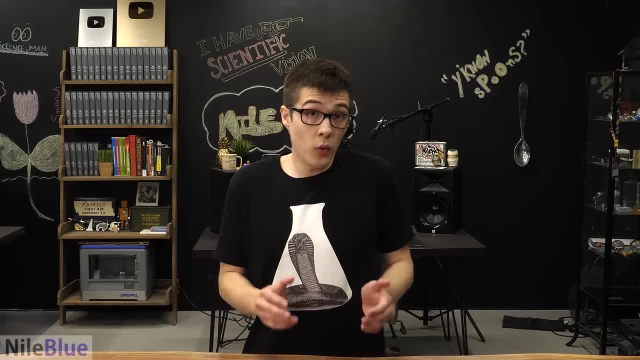 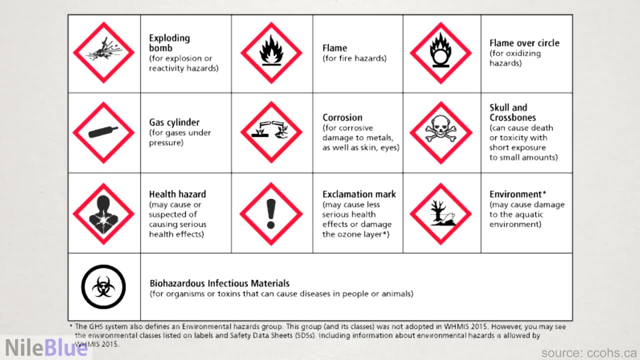 though, is the next layer, which is research. To avoid accidents or injuries, you fundamentally need to know what you're doing and all the risks that are involved. Before any project, I make sure that I know the properties and all the dangers of every chemical that I'm using and all the 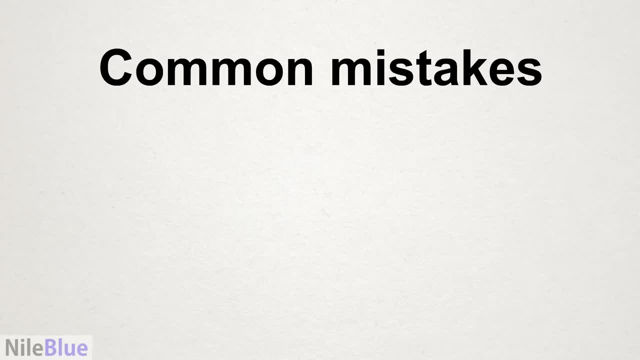 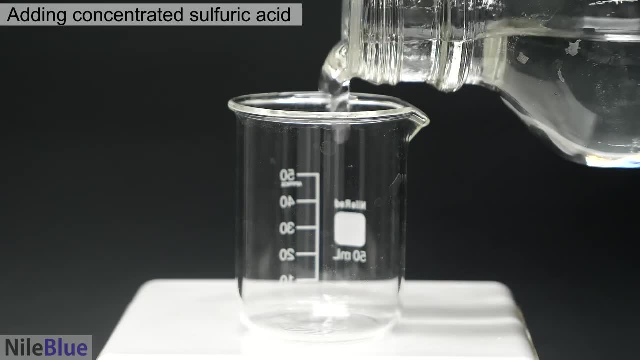 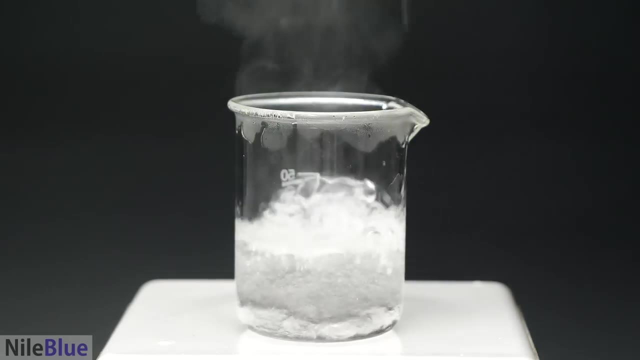 possible reactions that they might have. One of the most common mistakes is to accidentally mix some incompatible chemicals or to mix them improperly. Some of these mistakes are more commonly known like adding water directly to a concentrated acid. It can create enough heat to violently boil and splash stuff. 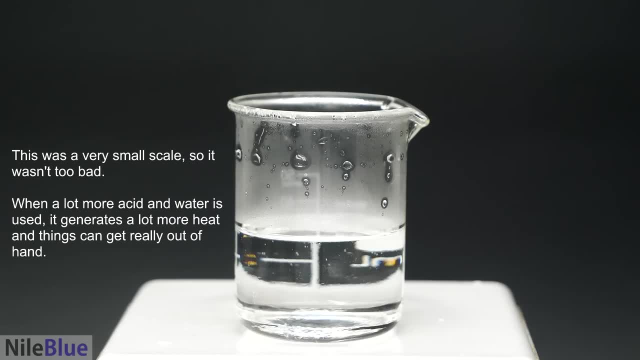 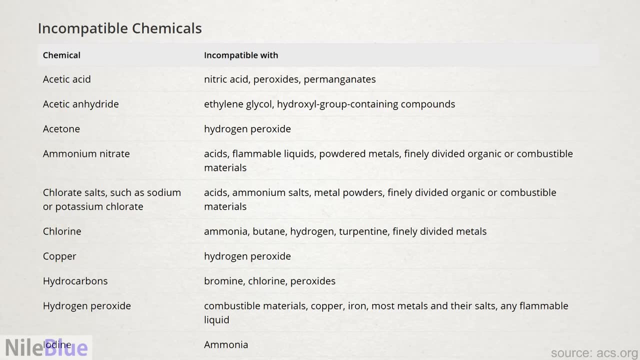 everywhere. When it's done the other way, so acid to water, it still generates a lot of heat and it needs to be done slowly, but it's much easier to control. The less commonly known errors, though, come from accidentally mixing together incompatible chemicals. This is a list of all. 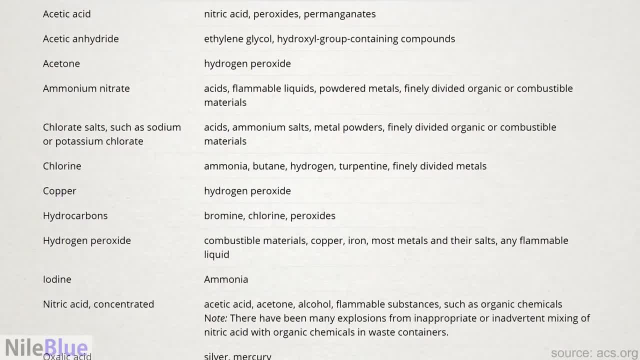 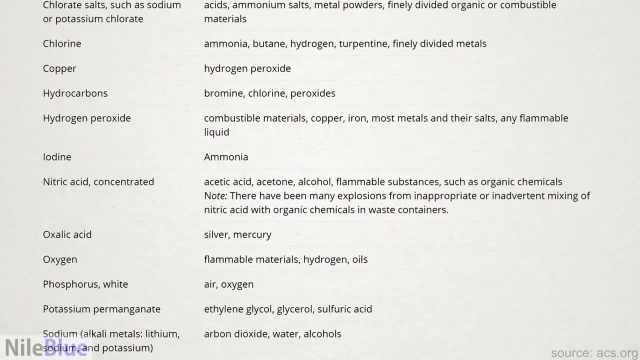 the common incompatibilities that I pulled from the ACS website and it shows the major ones to look out for. All the chemicals involved here are common lab chemicals and if they're mixed they can either react violently, become explosive or will. 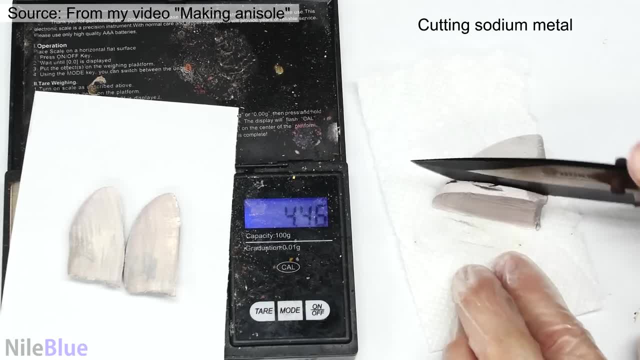 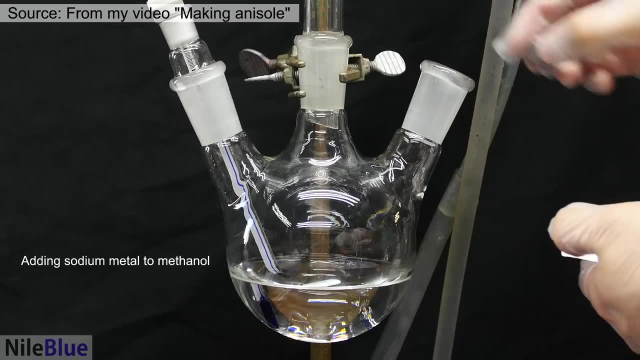 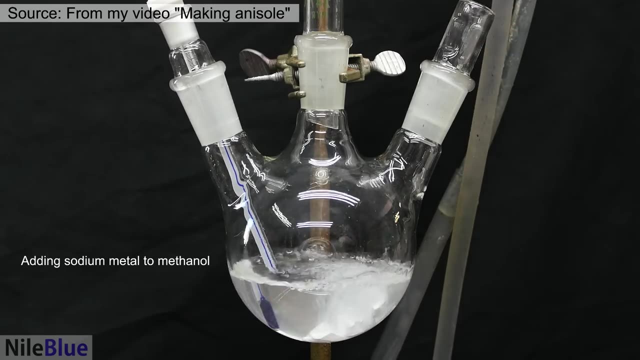 generate toxic or poisonous gas cause this to happen. What's interesting is that a lot of these combinations are able to be done safely, and they are sometimes done purposely. For example, for some chemical reactions, you need to combine sodium with alcohols, and I've done this a couple of times on the channel. I also 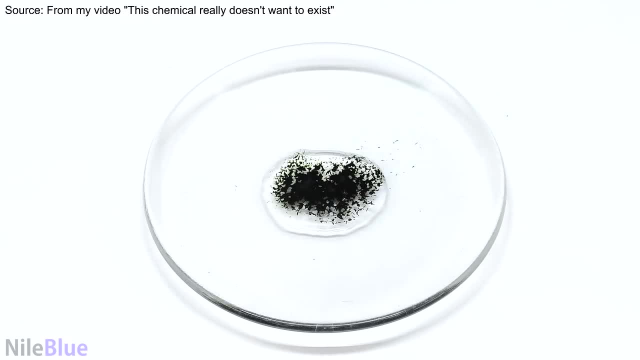 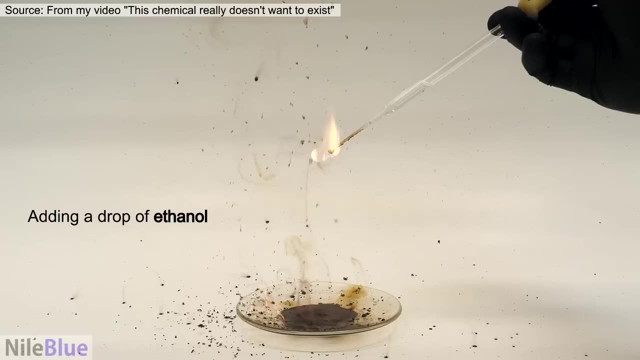 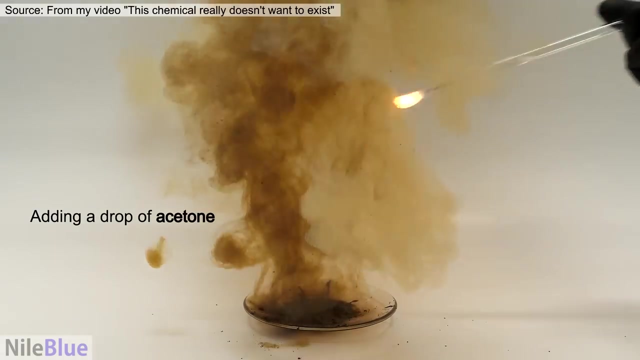 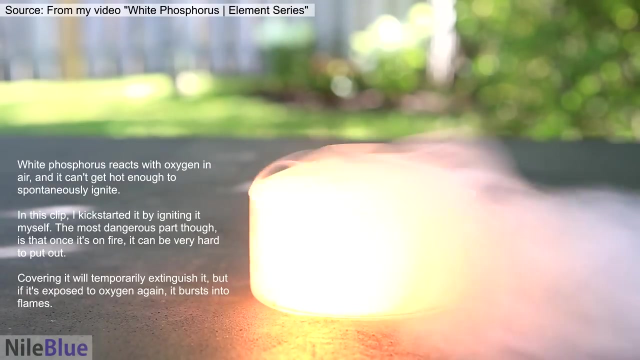 made a video where I combine sulfuric acid with potassium permanganate to make the really unstable manganese heptoxide. So it's not that you can never combine these chemicals- ever. it's that you just have to know what you're doing and be prepared to handle the reaction that will happen. 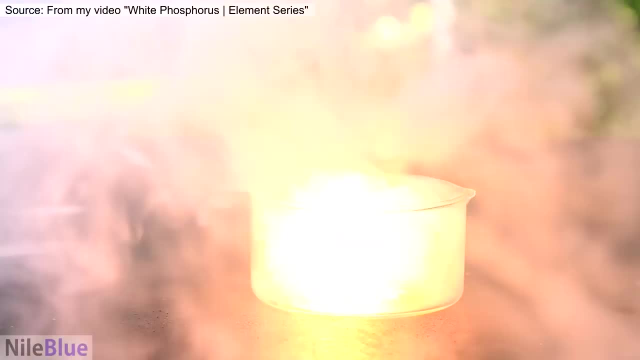 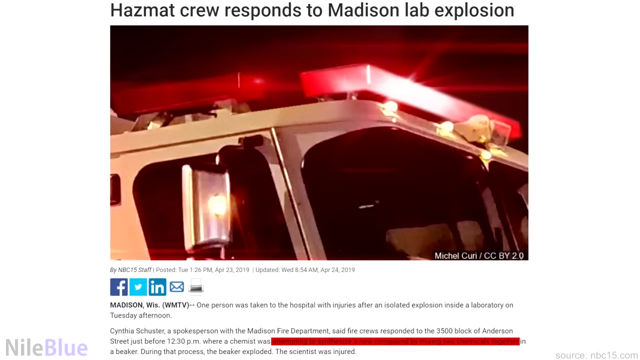 It's only when it's accidental and you don't expect it that it starts becoming dangerous. It's also really not uncommon to hear about lab accidents that were caused by mixing incompatible chemicals. It even happens in university research labs and in industry, where people have been trained. 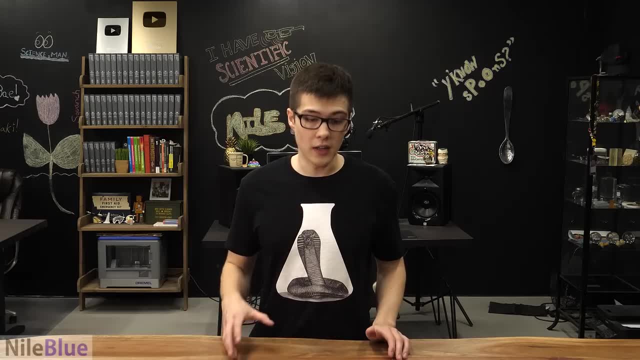 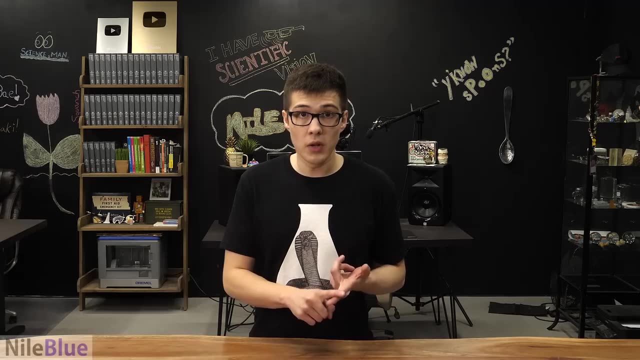 and they're supposed to know what they're doing. So before working on anything, I do a lot of research to know exactly how everything interacts and what could go wrong. For example, could it explode? Is there a risk of it bubbling out of the flask? 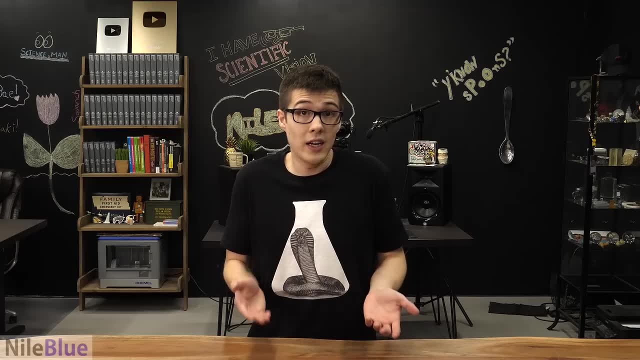 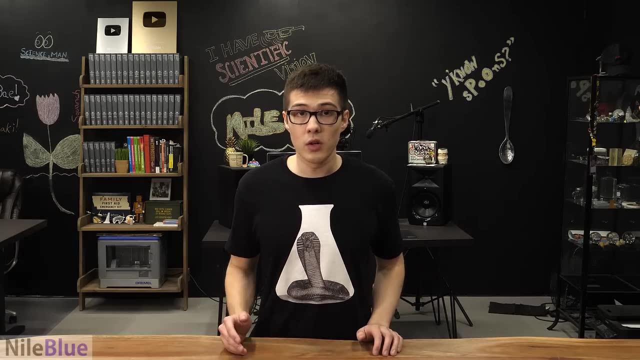 Could it light on fire? What if it spills? How would I clean it up? What if it gets on me? What safety protocols do I have set up for that? Even things like what if the power goes out and I have no light or my fume hood stops? 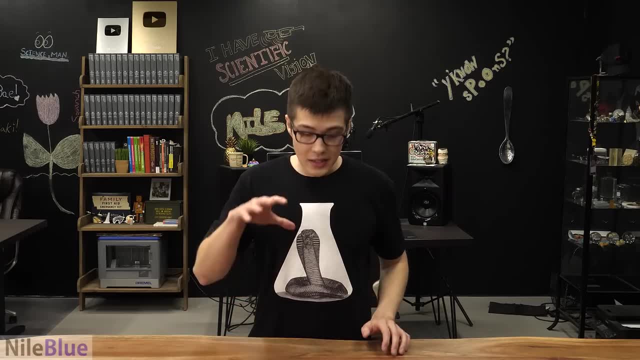 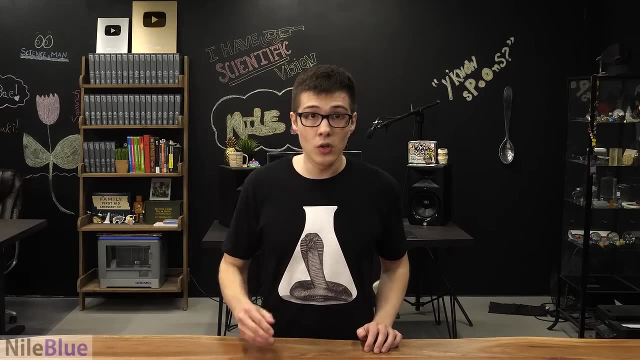 working. Then, after I think about all this, I take all the precautions to deal with all these possible issues. My general approach is to assume that the absolute worst thing will happen and to only start if I feel that I'm prepared to deal with it. 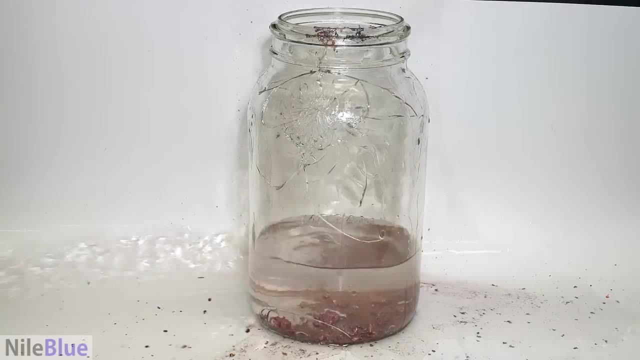 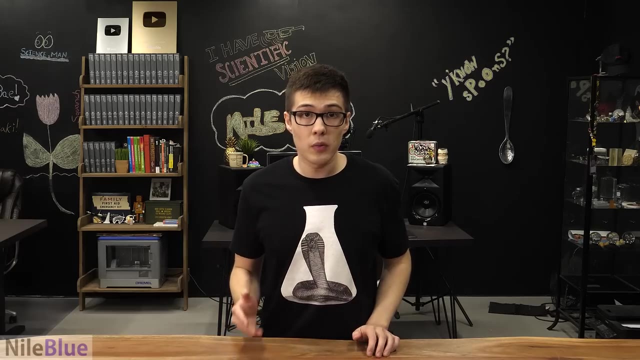 If I don't feel comfortable dealing with the worst possible scenario, then it's time to do something that I should be doing. This is not only for my own personal safety, but also for the people around me as well. If my worst case scenario at all involves potentially harming someone else, then the 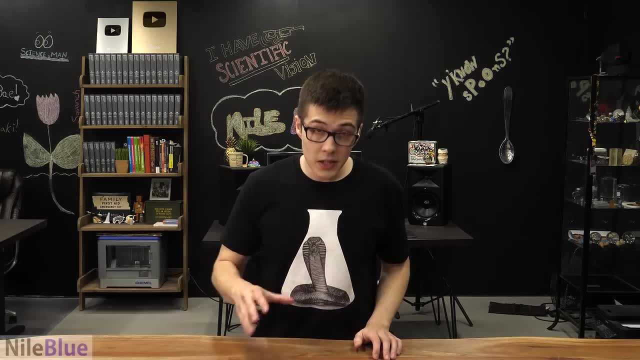 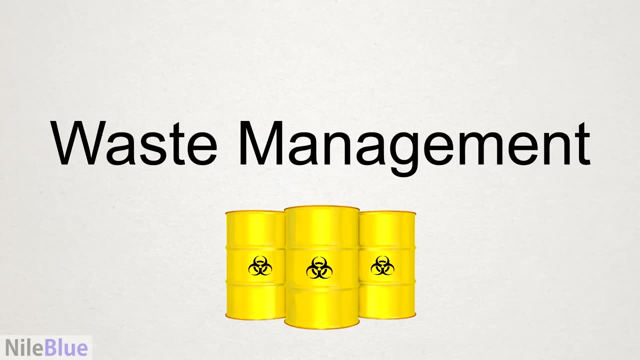 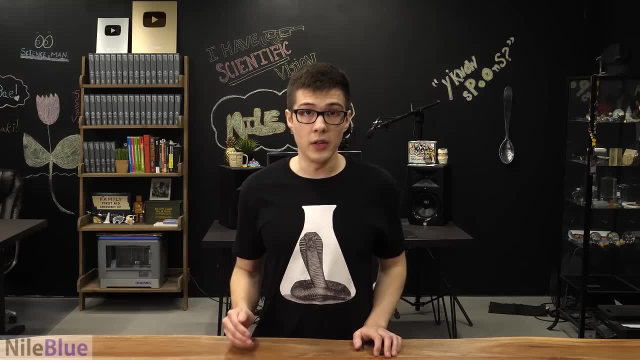 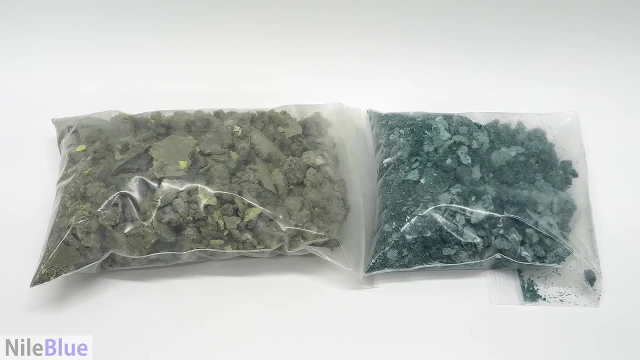 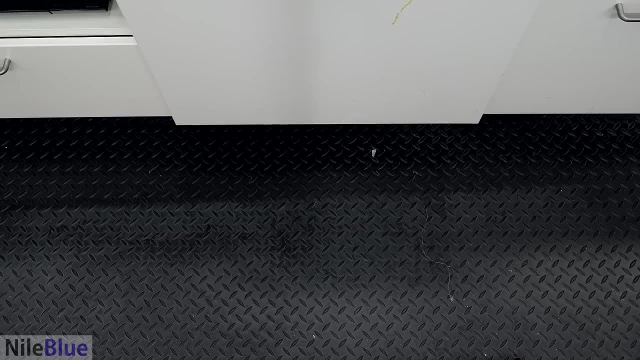 I haven't really been able to do that. I haven't really been able to do that. I haven't really been able to do that. I haven't actually made very much of it, but I will eventually have to pay a company to have it taken away. 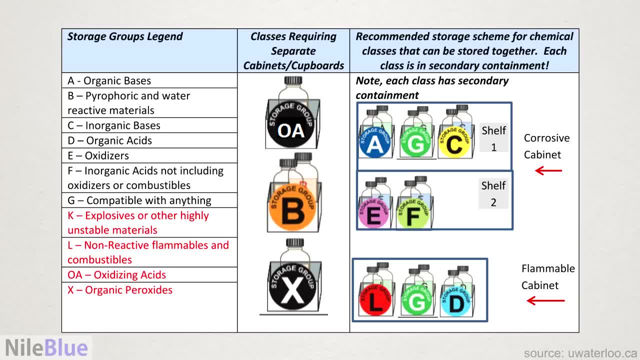 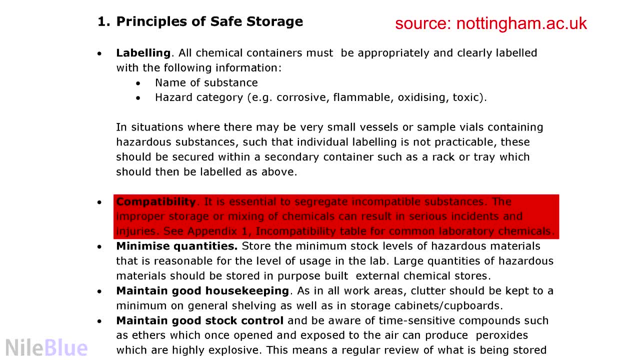 Another very important thing is how the chemicals are stored. Every chemical has different properties and everything needs to be organized in a way to minimize the risk of a reaction. The simplest form of this is to separate things like acids from bases and oxidizers from. 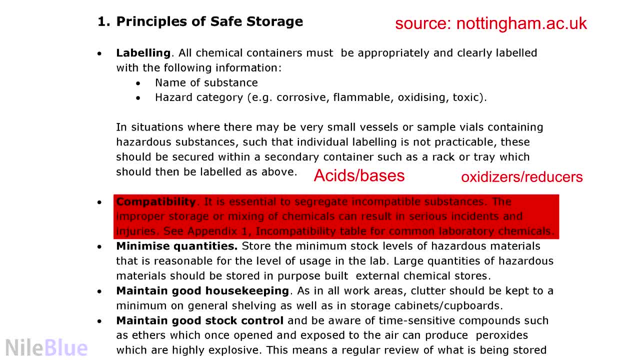 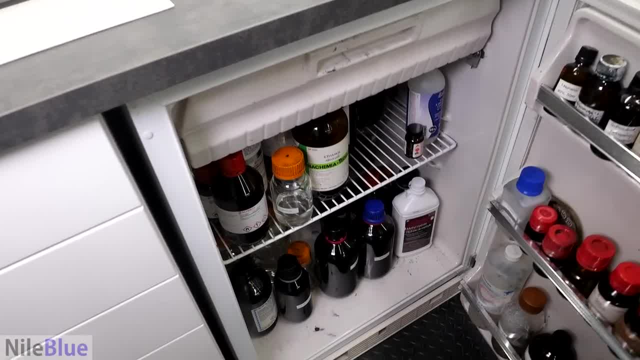 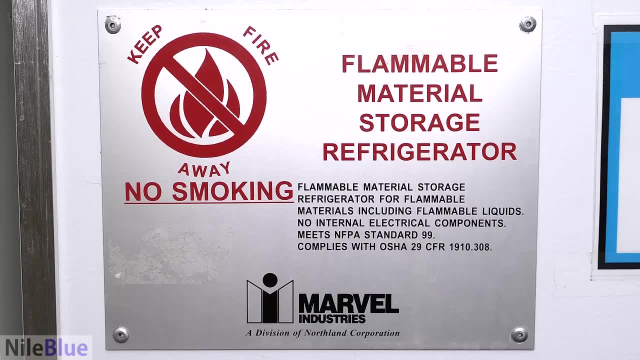 reducers and to keep them in completely separate areas. Flammables are also kept separate and some highly volatile or non-dense chemicals are, or unstable things are kept in a fridge. The fridge also has to be a specialized, explosion proof fridge that won't ignite any of the vapors when it tries to turn on. There have been many 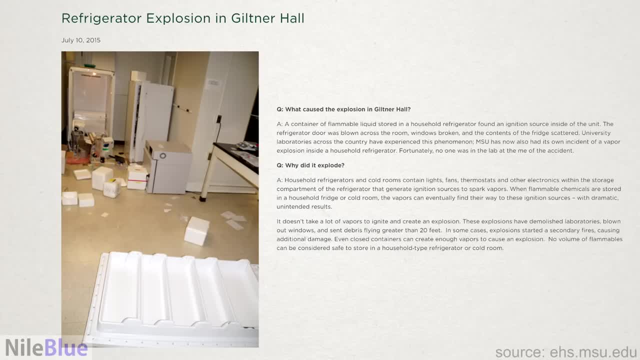 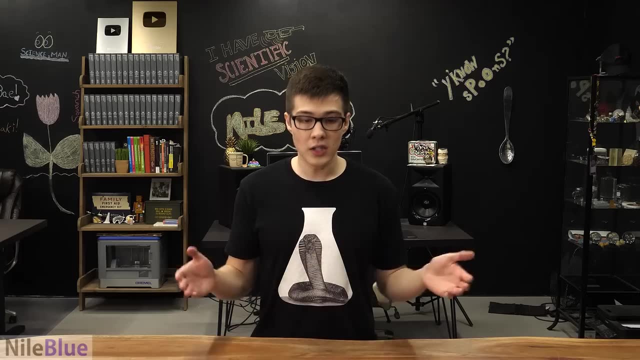 stories of fumes building up in just regular fridges and then, when it turned on, it ended up detonating. I could keep going on like this for a while, but the main point is that you can't just throw all the chemicals together in the same cabinet or something and assume that it would. 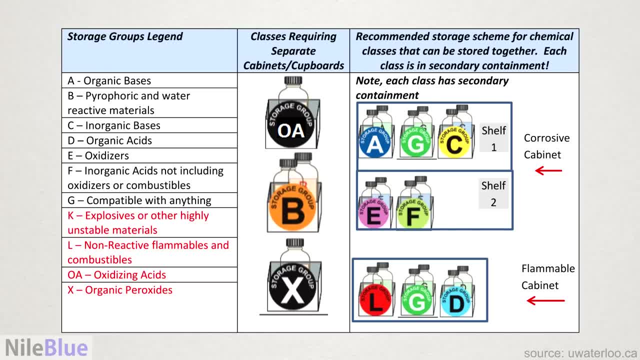 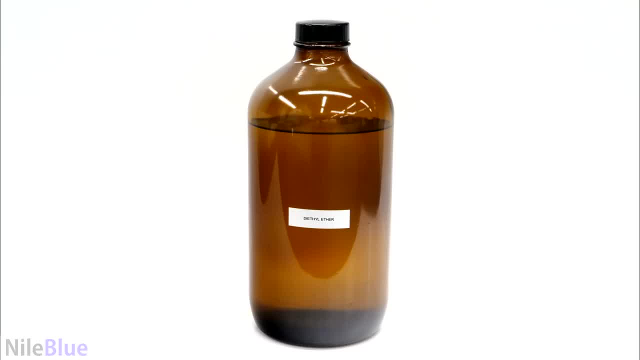 all be fine. Even if things are stored optimally, though, all the chemicals still need to be checked on frequently to make sure that they aren't either leaking or degrading. For example, some common solvents like diethyl ether or THF have a tendency to naturally form explosive peroxides. For this 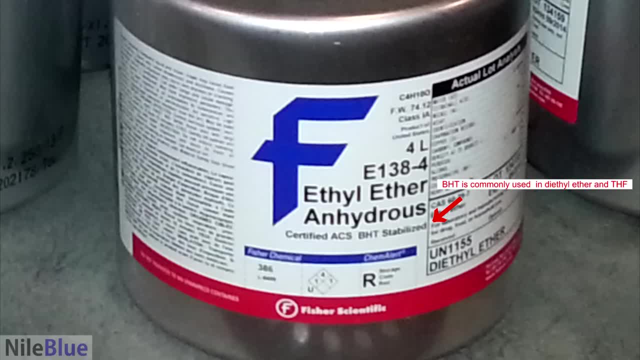 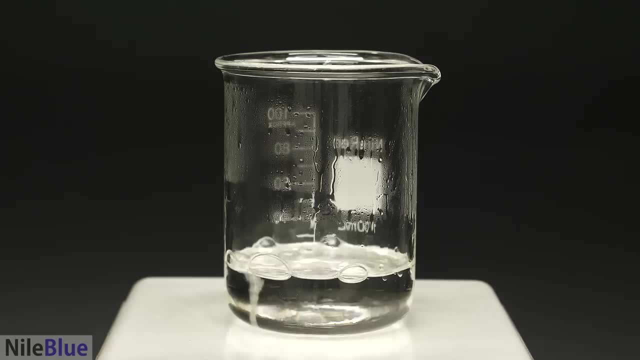 reason they're usually stabilized with something to prevent this, but even then they have to be monitored. Over time, even if it is stabilized, peroxides can start to become more and more explosive and then, if the solvent is evaporated, it can cause them to detonate. Like I said before, 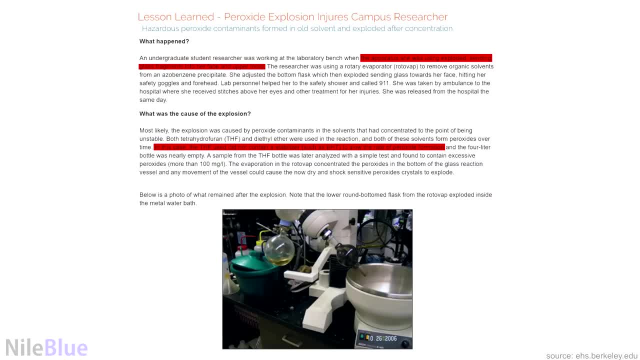 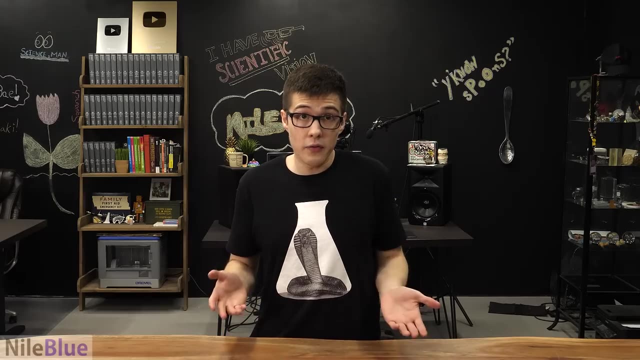 about incompatible chemicals. it's not uncommon to hear stories about this happening and causing an explosion. Also, the worst part about chemistry is that because everything's done in glassware, all the explosions involve a lot of glass shrapnel. And now the last thing is just behavioral and 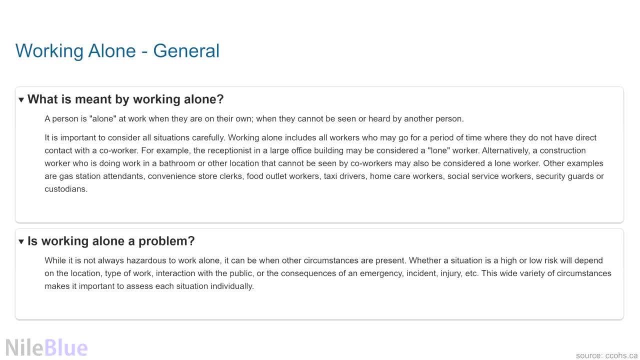 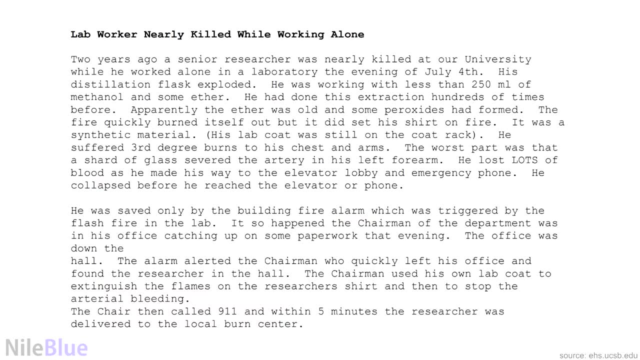 there are a lot of miscellaneous rules. The first is to be very careful about working alone and to inform those around you what you're doing. There have been many sad cases of people getting injured or killed because they were working alone. This doesn't mean that you can never work alone, though. 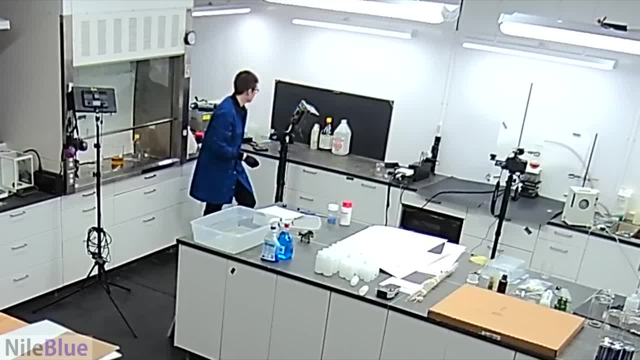 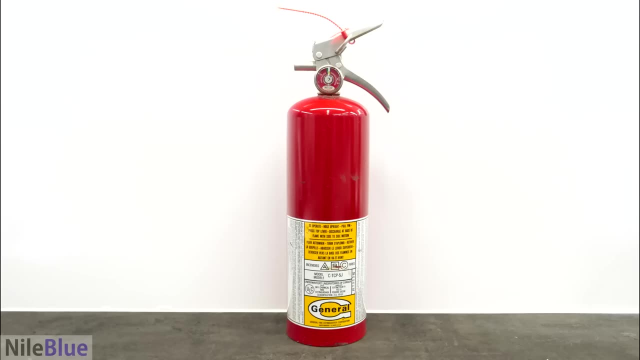 and it just means that you need to carefully assess the danger of what you're doing and know if it's okay to do on your own. Some things are totally fine to do, but sometimes you need to have other people around you who are able to help. if there ever is an emergency, These people should. 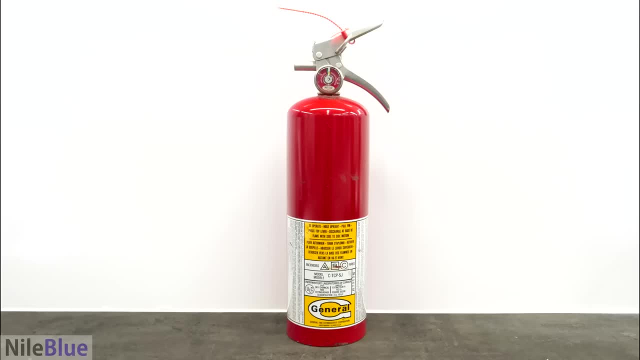 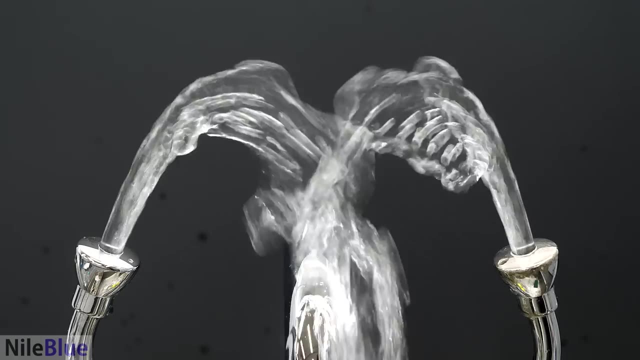 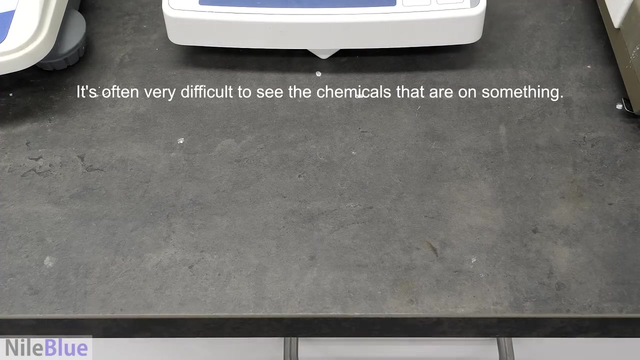 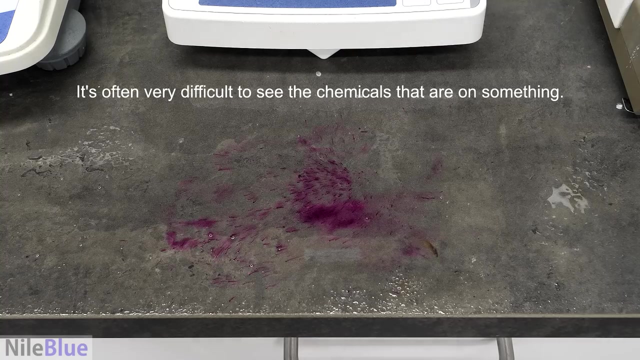 also be briefed with a lot of information about what you're doing and what you're doing. If you're in the lab, you should act as though every surface is contaminated. So the moment you touch pretty much anything, you are no longer able to touch your face, your phone or your clothing. 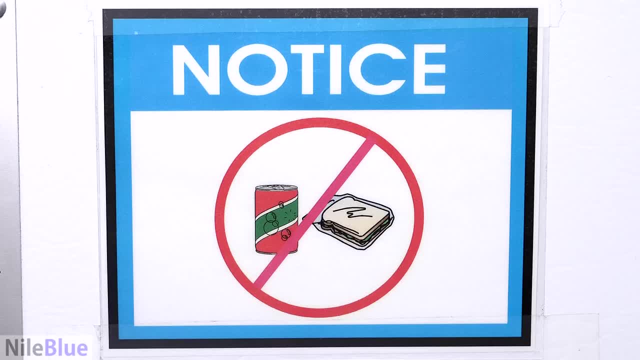 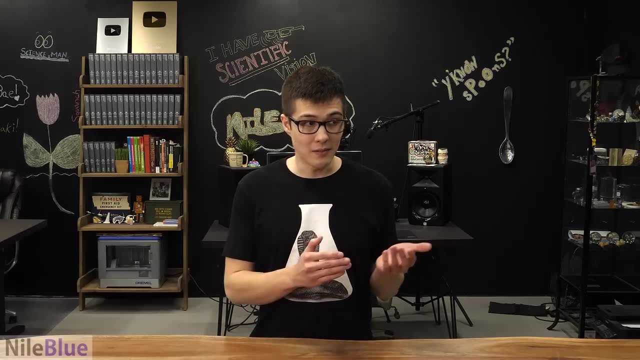 in general, You should never eat in the lab either or bring in any form of food. Almost everyone has made the mistake of being distracted and then drinking from the wrong cup, and I don't really think I have to explain why that would be a problem. Also, food would just get contaminated. 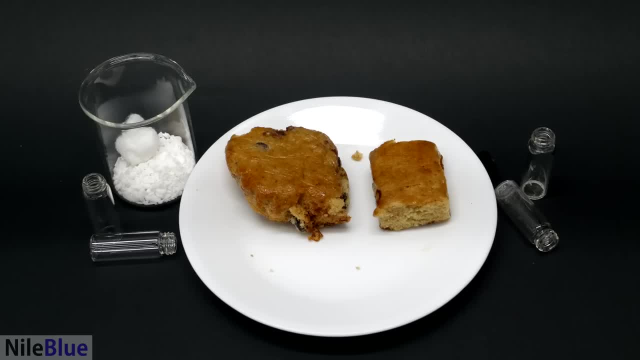 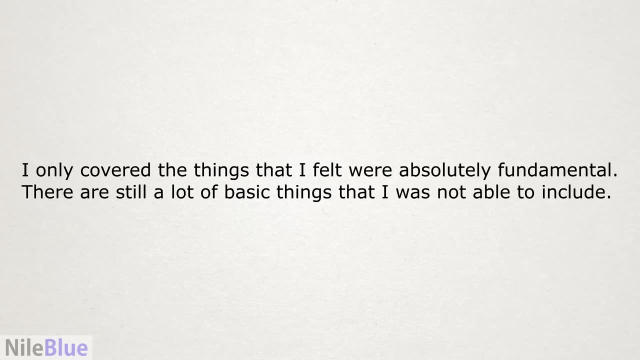 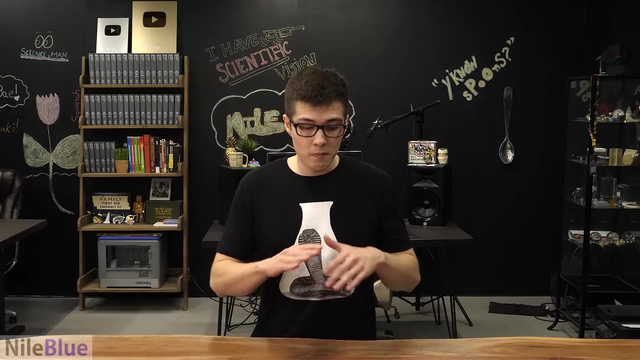 in general, and this is the easiest way to spice your food with chemicals. But finally, with all of that being said, I think that I covered most of the basic safety things when it comes to chemistry. However, I do want to be clear that this was not at all comprehensive and 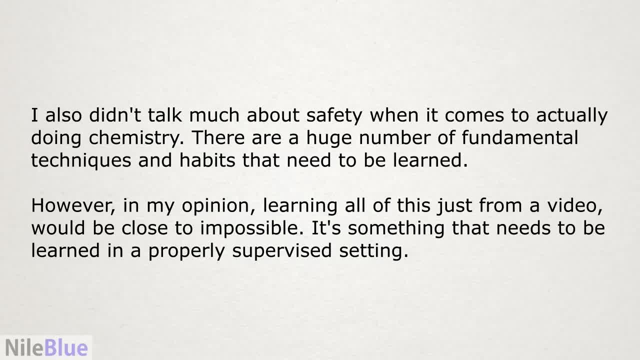 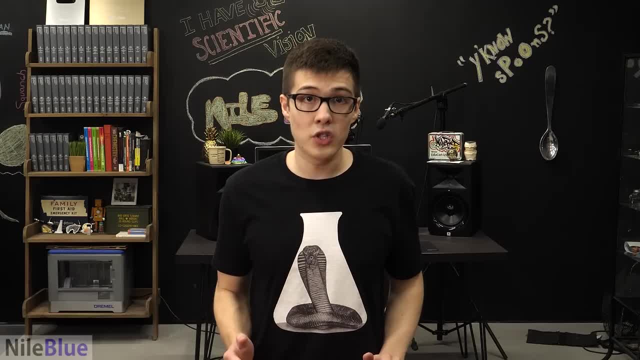 there's still a lot of stuff that I didn't include. Also, knowing these basic rules isn't going to be enough to just jump into doing chemistry, especially as an amateur or hobbyist. Before starting the Niall Redd channel, I had years of experience as a science student. 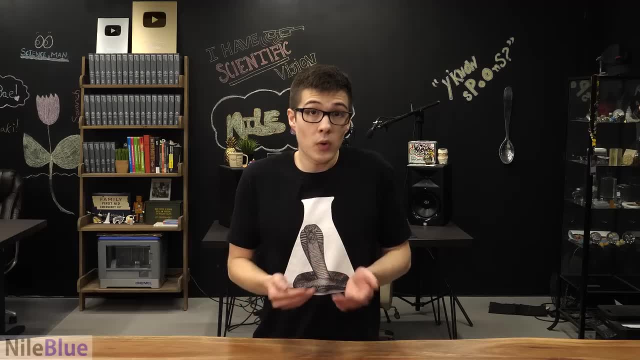 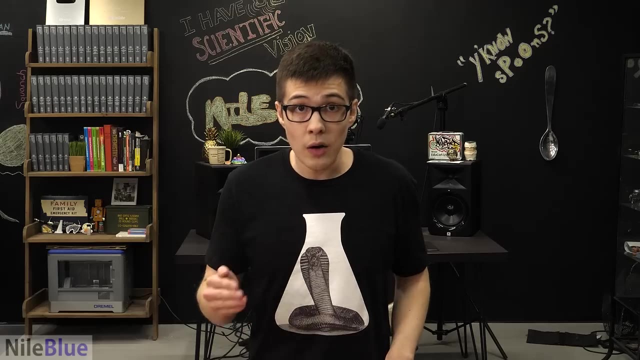 and then as a lab tech and a grad student, before I even attempted it on my own, And even after all that, I feel like I was just barely competent enough to do it safely. This is because to do it yourself, you not only need to know all the safety protocols, but also how to set them up. 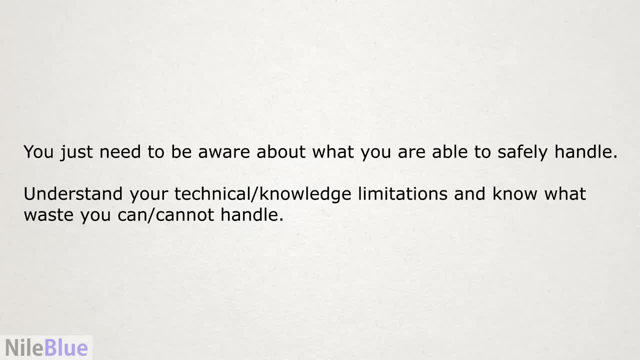 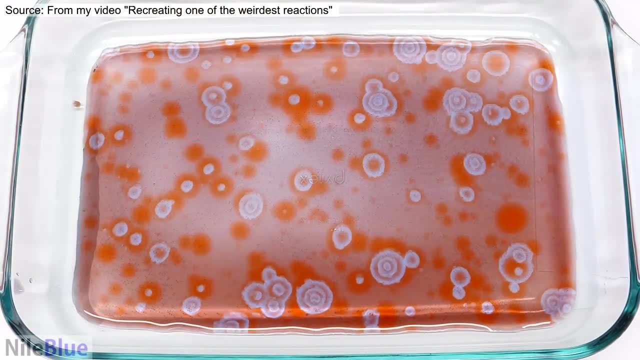 properly. This isn't to say, though, that it's absolutely impossible to do chemistry on your own at home. There are a lot of projects that are totally fine to do because they only need basic PPE and they don't produce any waste that's difficult to deal with. Some examples of this: 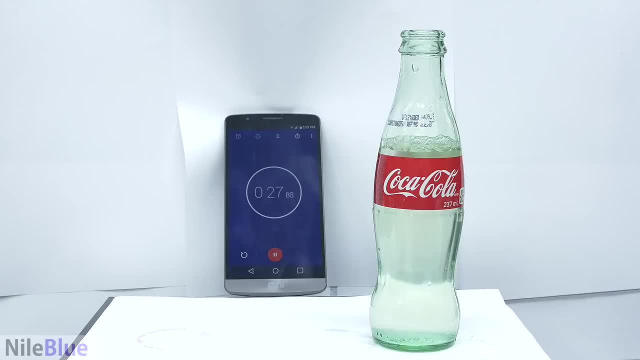 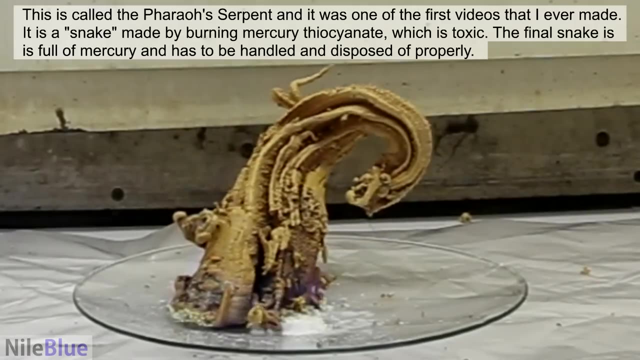 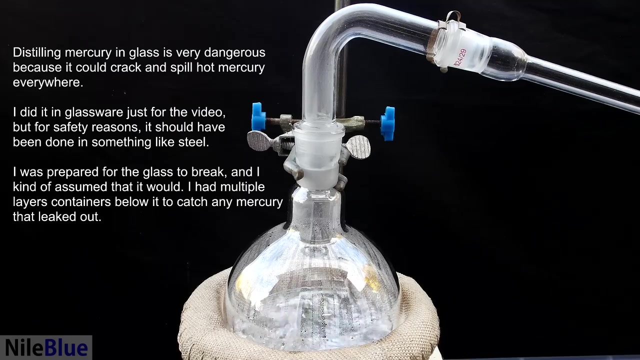 might be things like extracting DNA from strawberries, the iodine clock reactions or growing tin crystals. However, there are a lot of projects- probably most of the ones that are on my channel- that would be a lot harder to do safely and responsibly. For example, distillations of 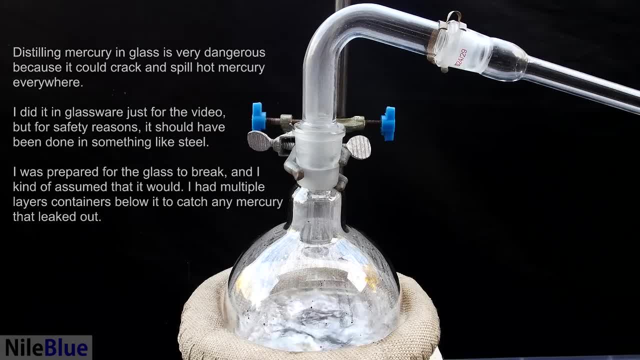 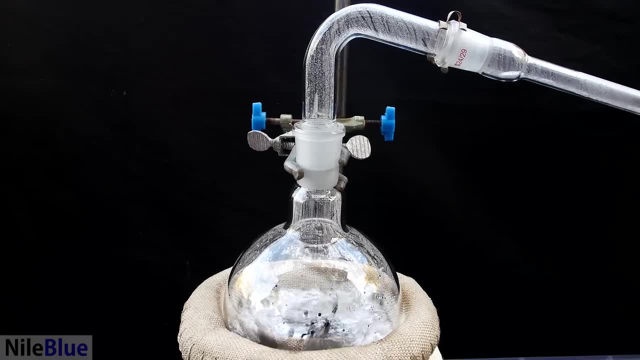 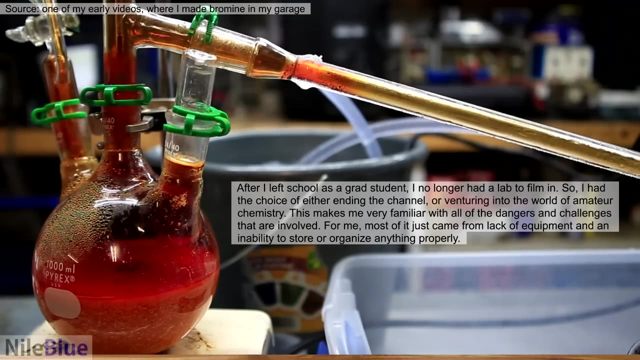 things like mercury, metal or sulfuric acid are insanely dangerous, and just wearing standard PPE and thinking it's all going to be fine is a recipe for disaster. This is one major reason why amateur or hobbyist chemistry has always concerned me a bit, especially because it's 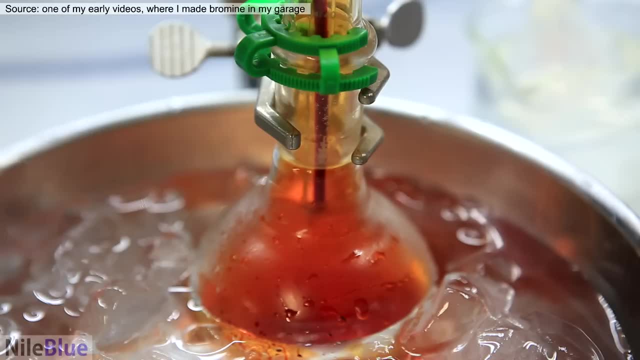 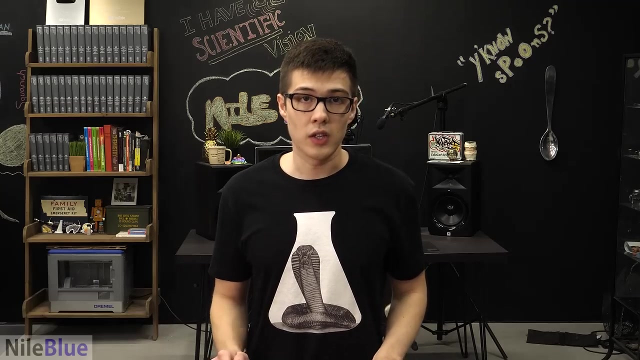 something that is implicitly promoted by my videos. I genuinely believe, though, that without some form of proper training, it's just not possible to safely do a lot of it. Chemistry is fun and exciting, but there is a very real danger to it, and that can never be overlooked. 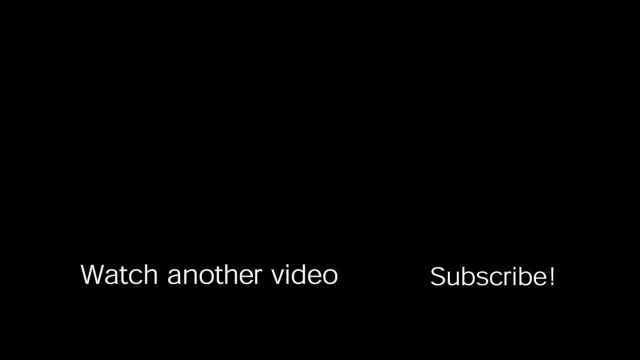